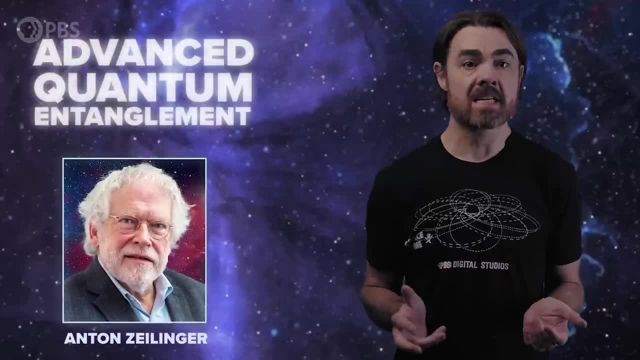 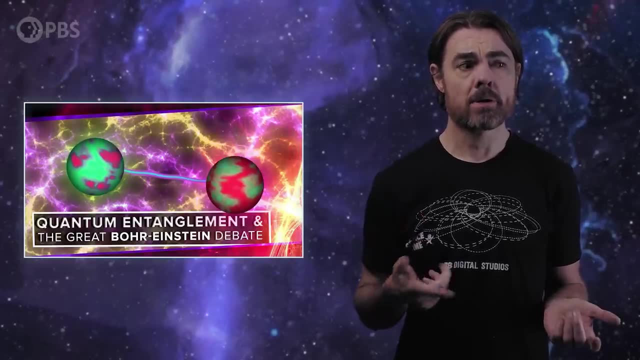 wrong, while Zeilinger greatly advanced our understanding and practical application of the phenomenon of quantum entanglement. Of course, we've talked about quantum entanglement once or twice in the past, But today I want to tell you about a series of brilliant experiments. 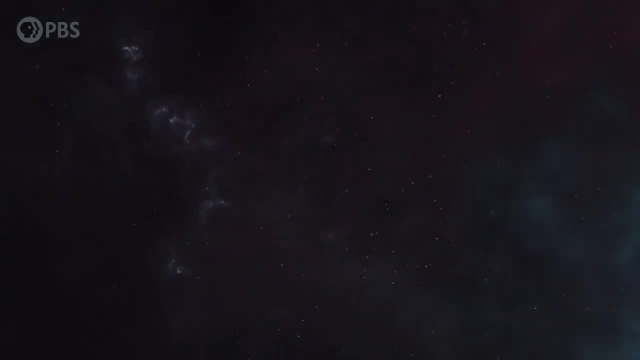 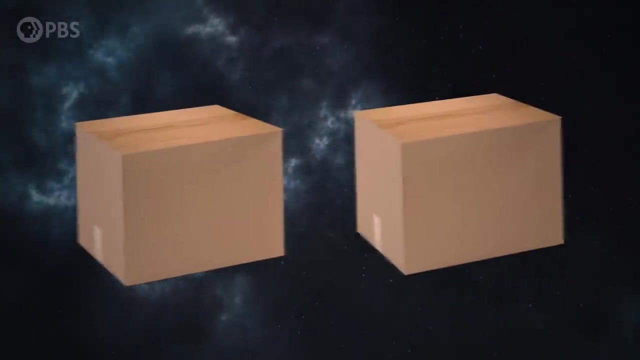 celebrated by this year's Nobel. Let's start with a simple thought experiment. You have two balls, One black, one white. You close your eyes, shuffle the balls and place each in an identical box. You put the first box in a rocket and send it to the moon. 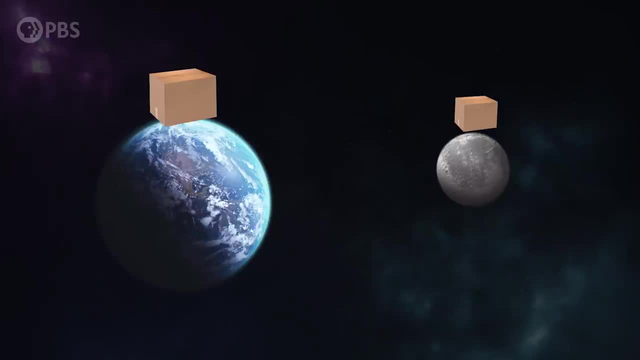 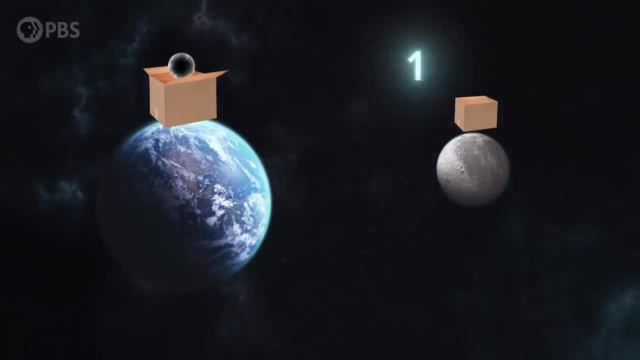 While you keep the second box with you on Earth. While that box is closed, the ball on the moon has a 50-50 chance of being black or white. You open your box and you instantly learn the color of the ball on the moon. 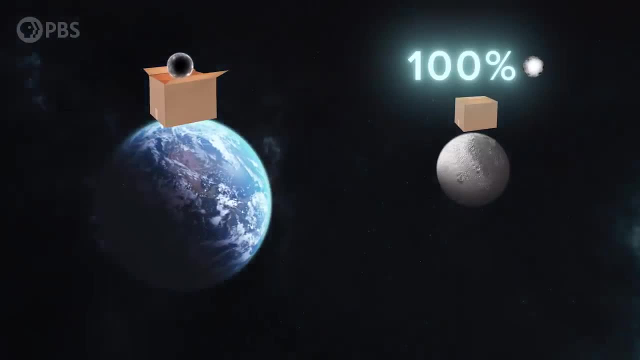 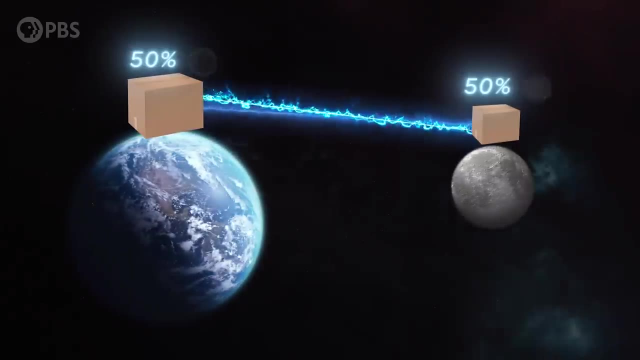 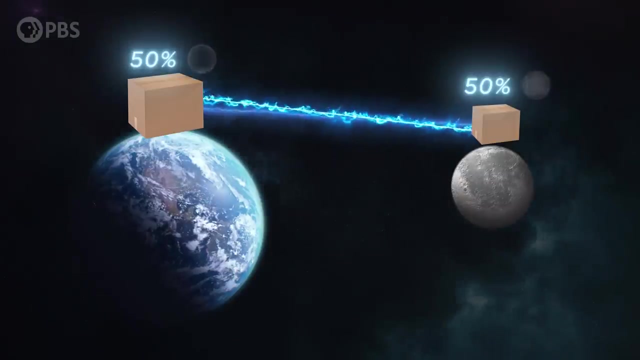 So did you cause information to travel faster than light? Of course not. The information about the balls' colors was always there with the balls. You just learned which was which, But now imagine that these are quantum balls with entangled quantum colors. According to quantum mechanics, we not only don't know which is which until the box. 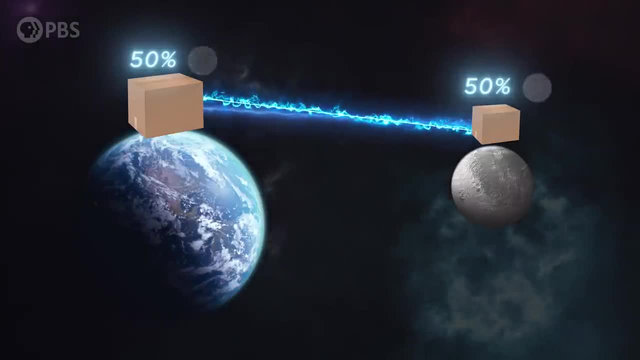 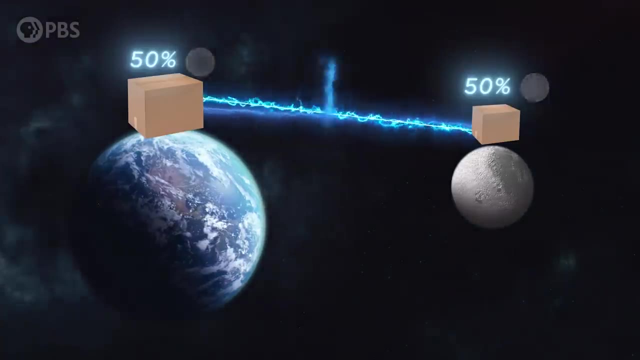 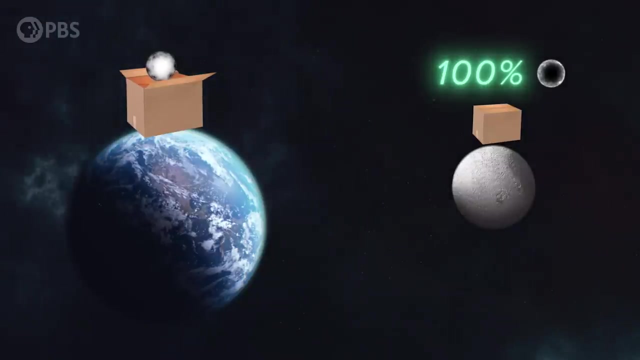 is open, but the colors of the balls are fundamentally undefined. Each ball is in a superposition state of maybe black, maybe white, until a measurement is made. Opening your box causes the observed ball to have to choose a color state, which then forces the ball on the moon to choose the opposite. 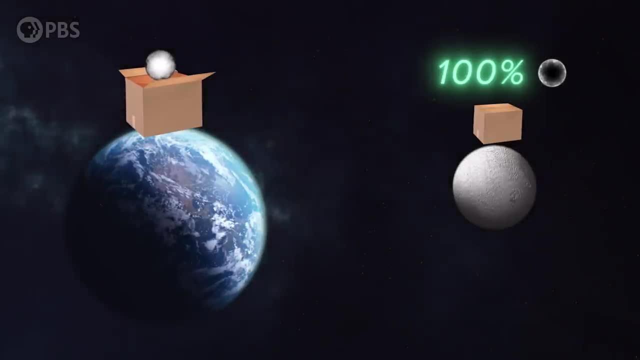 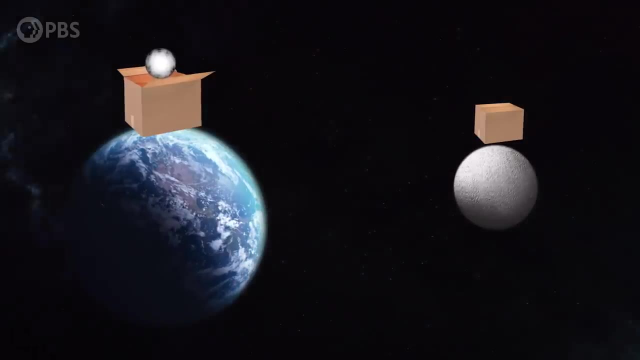 Now you really do seem to have an effect that travels faster than light, with the ball on the moon switching from a superposition state to a defined state as soon as you make your observation. These quantum balls could be any particle, from subatomic to molecular scale, and the 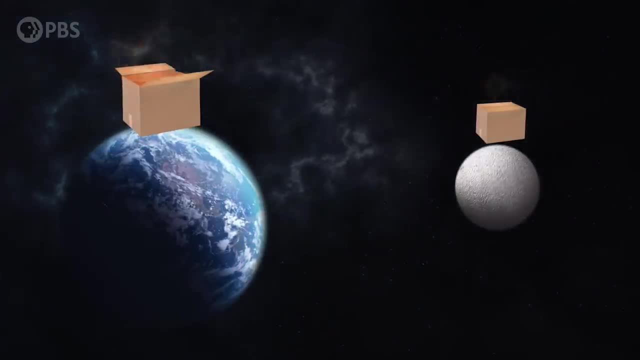 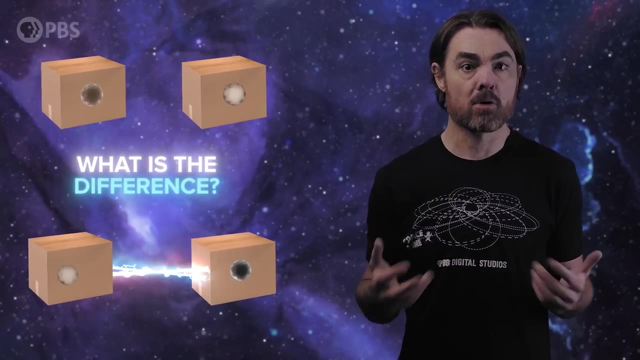 entangled property could be spin, momentum or any other quantum property. But why do we have to accept this wacky interpretation? Is there any real difference in the result of the experiment if the color of the balls is defined at the beginning versus when the box is open? 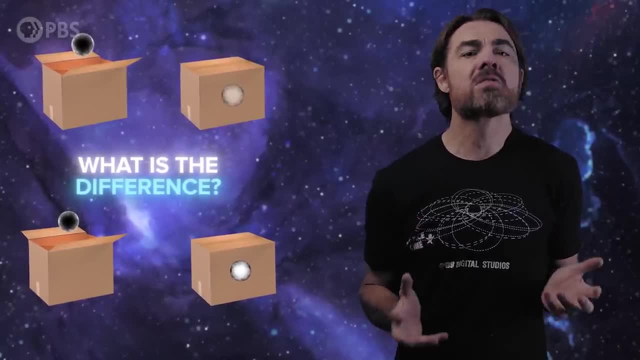 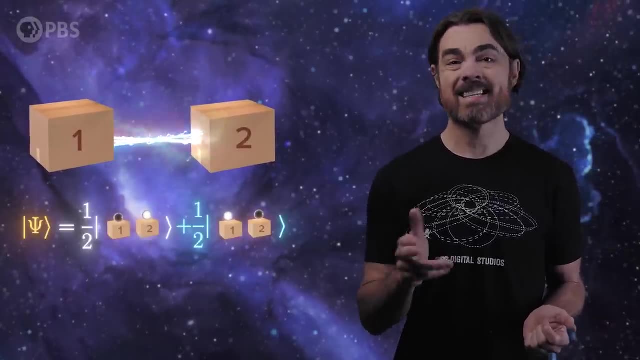 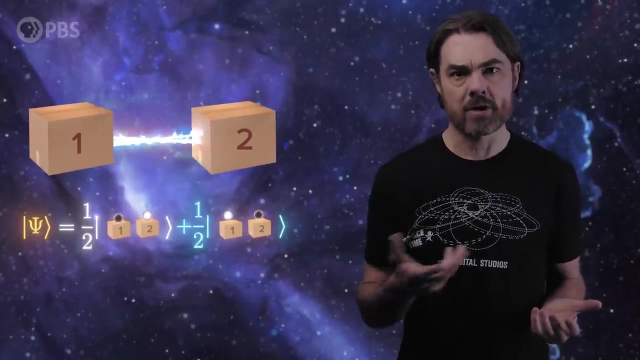 Or is it just a matter of time? Why even propose this entanglement and superposition stuff? Well, because quantum mechanics in its standard form says so. Quantum systems are described by a mathematical object called the wave function, which evolves according to the Schrodinger equation. 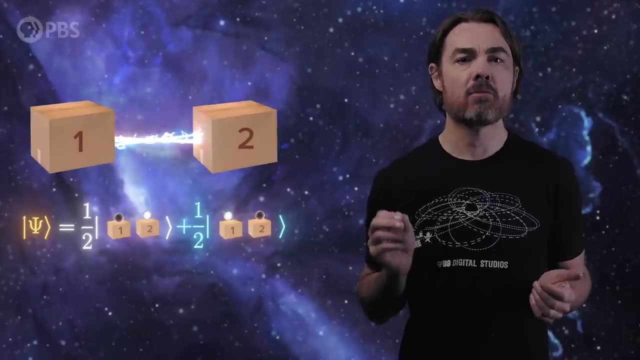 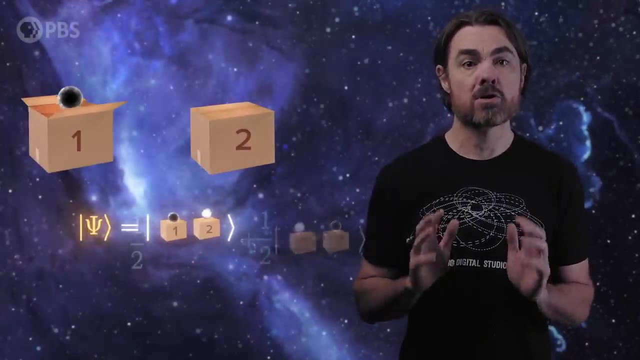 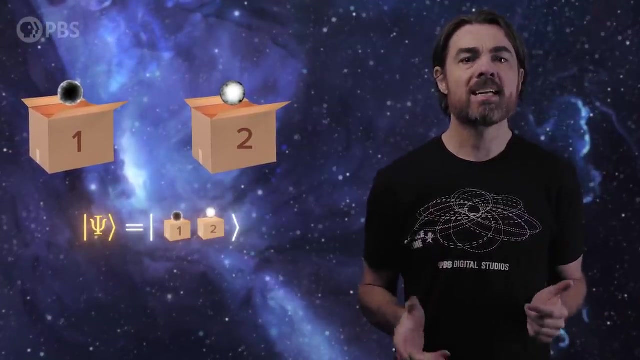 The joint wave function of two entangled objects only contains information about the correlation between those objects, not about their specific values. They only gain specific values when observed And the wave function collapses. For our quantum balls to know their own color the whole time, there would need to be extra 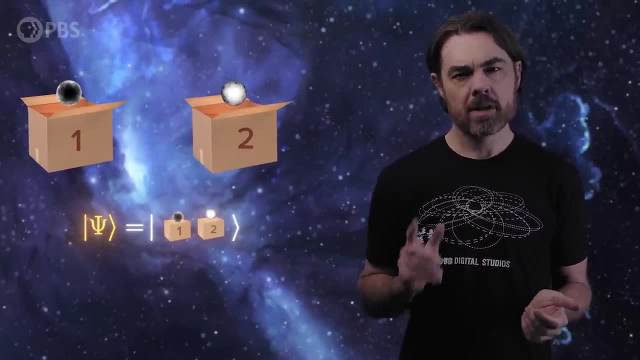 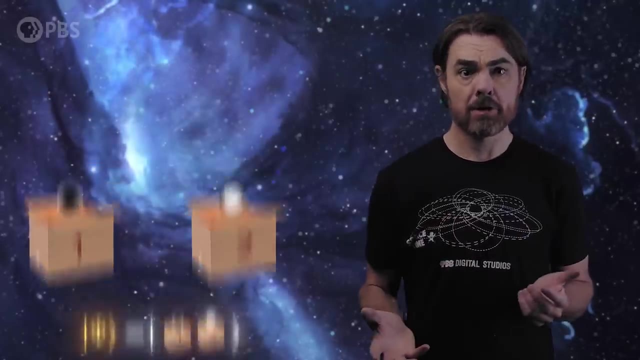 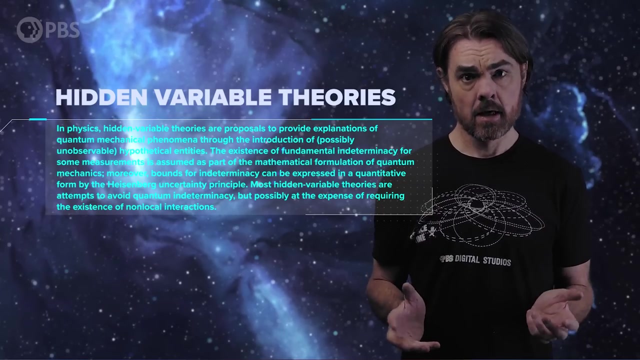 information not contained in their wave function. There are a few different interpretations of quantum mechanics that allow this hidden information, and they are collectively known as hidden variable theories. Einstein thought that such hidden information must exist, while others, like Niels Bohr, insisted that the wave function was the complete dissonance of quantum mechanics. 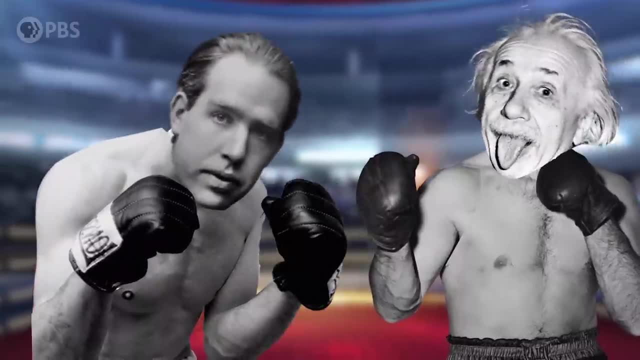 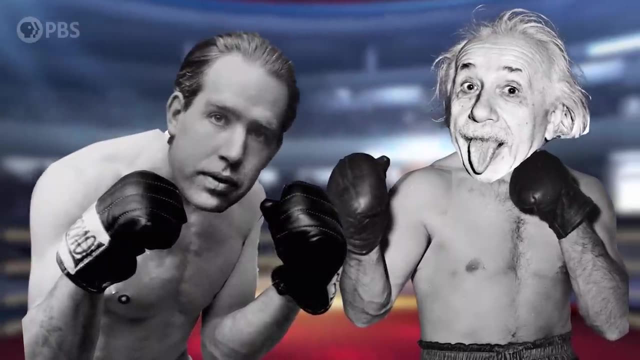 This is why the wave function is so important. It's a complete description of a quantum system. In almost every scientific debate, physicists side with Einstein, But not in this case. Quantum mechanics was just too successful and Niels Bohr was aggressive in pushing his 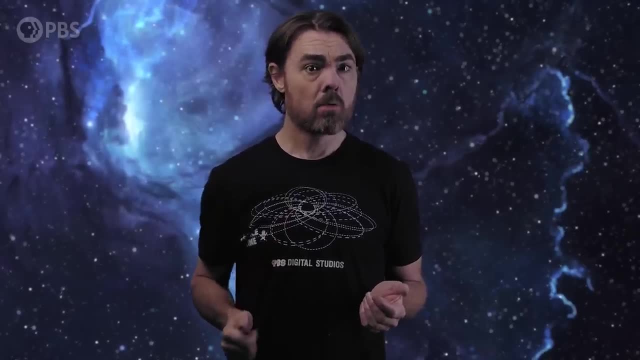 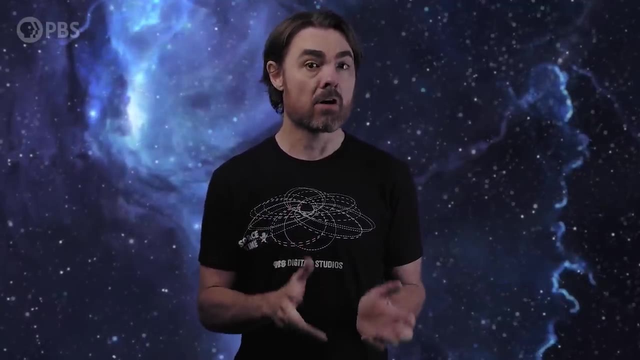 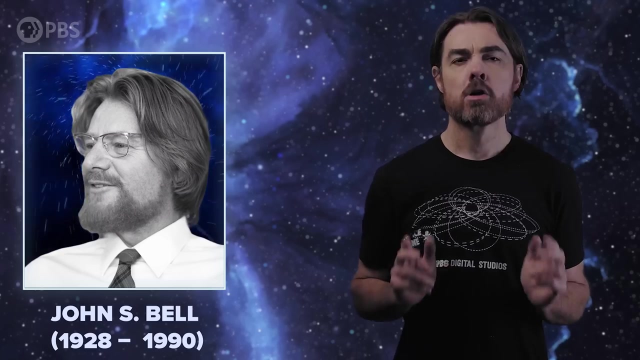 Copenhagen interpretation. It became dogma, while for a while it was career suicide to question the orthodoxy, For example by researching hidden variable theories. David Bohm got the worst of that with his pilot wave theory, Which we talk about in another video. 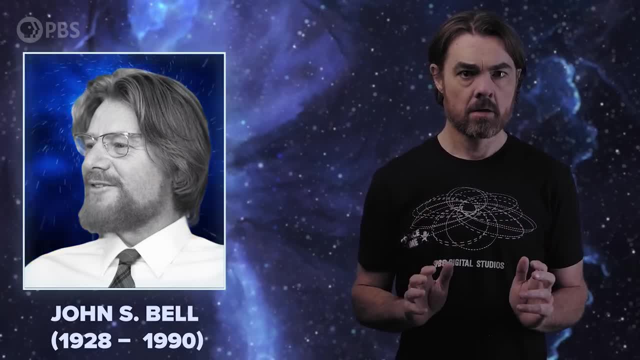 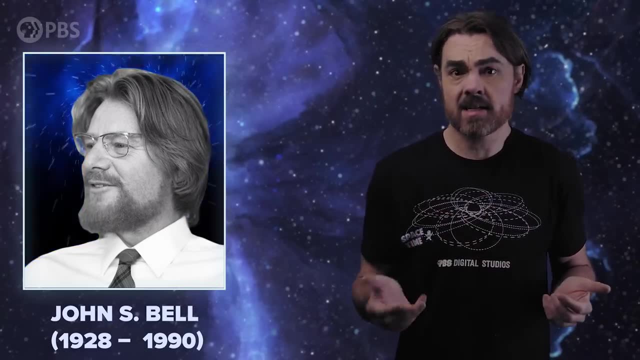 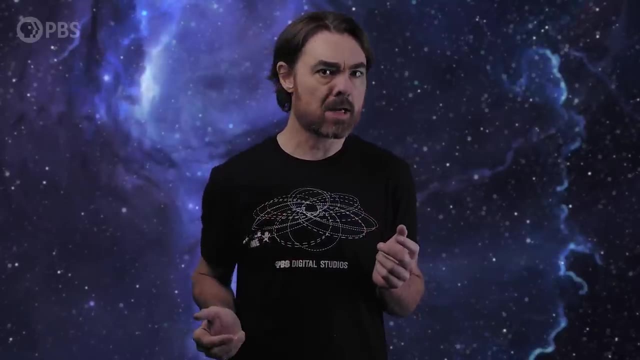 John Stuart Bell was another hidden variable heretic. This Irish physicist didn't necessarily believe in them, but he wasn't content to just accept the Copenhagen interpretation without properly testing it, And he also realized that one could reveal the existence of hidden information without actually measuring that information or even testing a specific hidden variables theory. 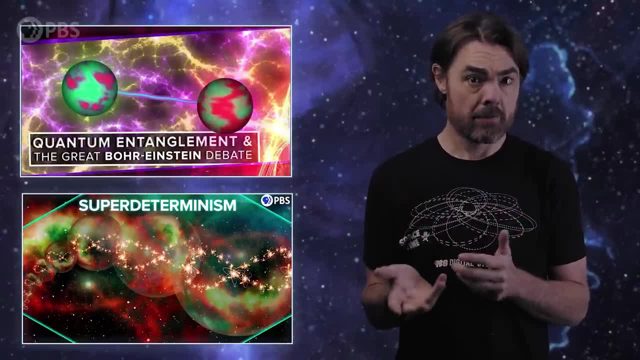 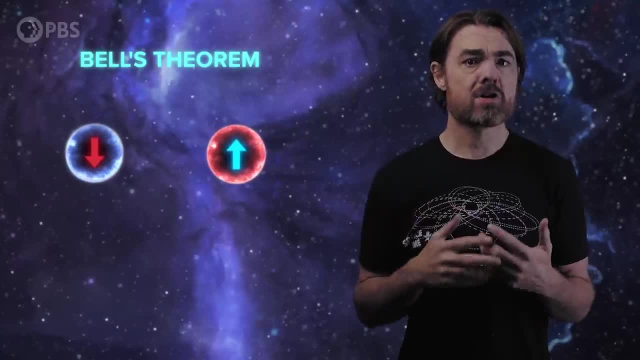 We've talked about these Bell tests previously, if you want to see exactly how this works. In short, though, in 1964 Bell came up with his Bell theorem, which shows that there should be a particular statistical correlation between the measured properties of entangled 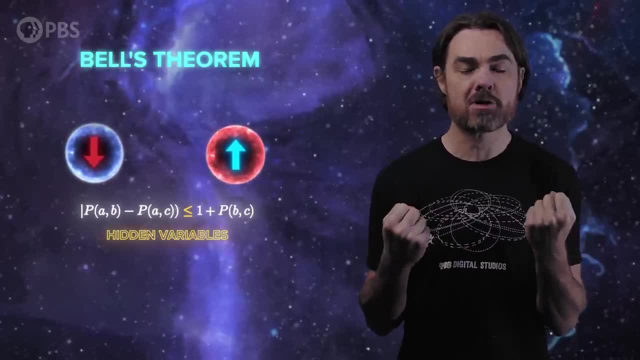 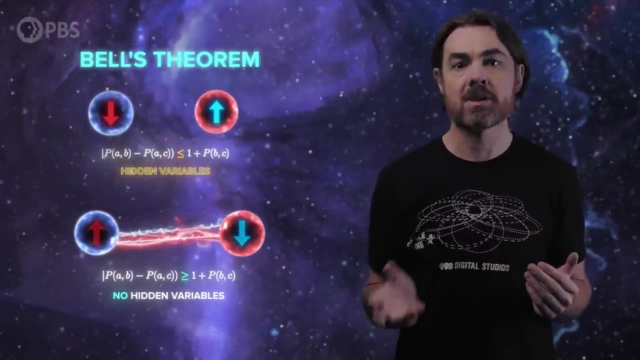 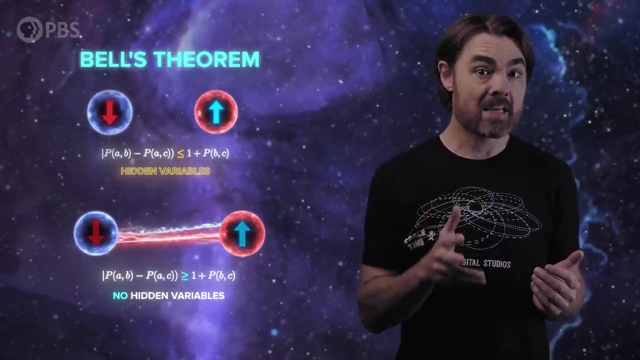 particles, if the particles themselves hold the information about their internal states and a different statistical relationship if those properties really are decided at the moment of measurement. In particular, the so-called Bell inequality would be true if there are hidden variables contained in the particles. 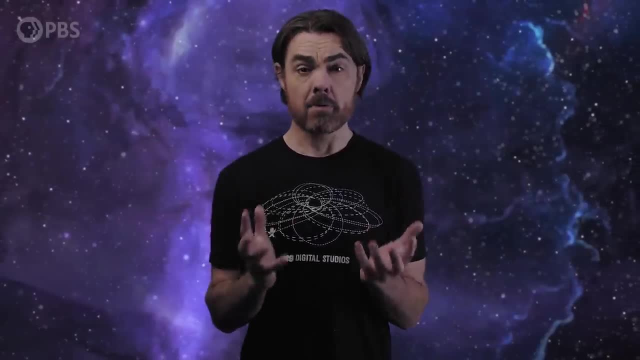 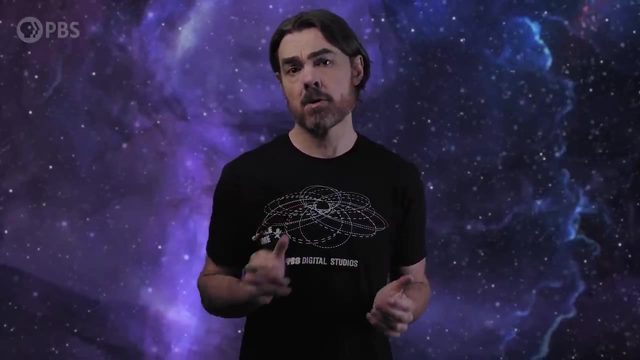 But that's not all. There was a real test that we could use to check for hidden variables. However, it wasn't until 1969 that the first Bell test was performed, and that was by one of our 2022 Nobel laureates, John Clouser. So why did it take five years? Well, Bell tests are really hard to perform. They require the production of entangled states which have to be manipulated and measured without breaking the exceedingly delicate correlation between the particles. But also, to do a Bell test was to question the status quo, so it was hard to get support. 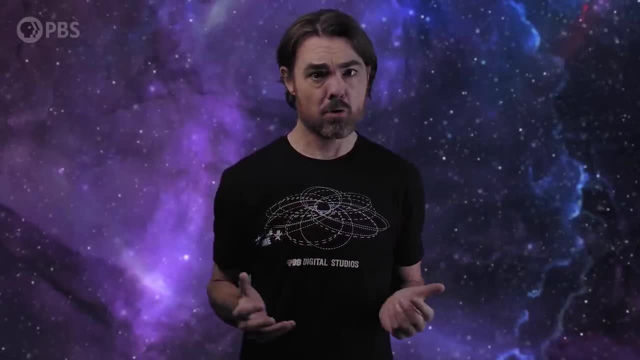 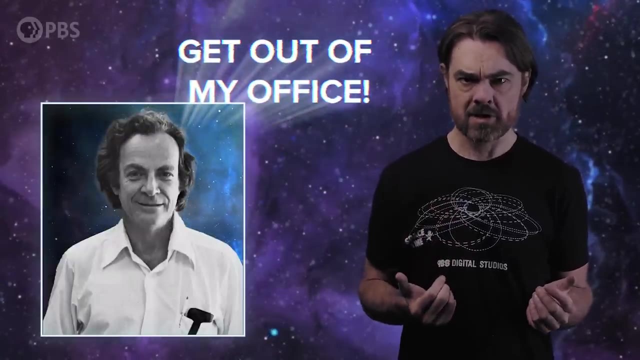 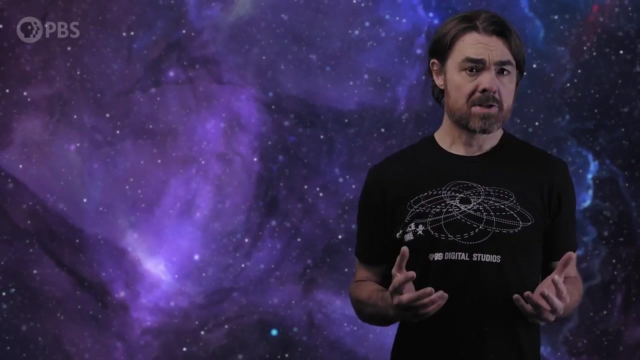 for the significant effort required. Clouser talks about the time he proposed his idea for the experiment to Richard Feynman, who promptly kicked him out of his office. Apparently, Feynman thought it was pointless, because standard quantum mechanics was clearly correct. Clouser and his student Stuart J Friedman were not to be deterred. They had figured out that there was no way to solve the problem of entangled states and that there was no way to solve the problem of entangled states. Clouser and his student Stuart J Friedman, were not to be deterred. 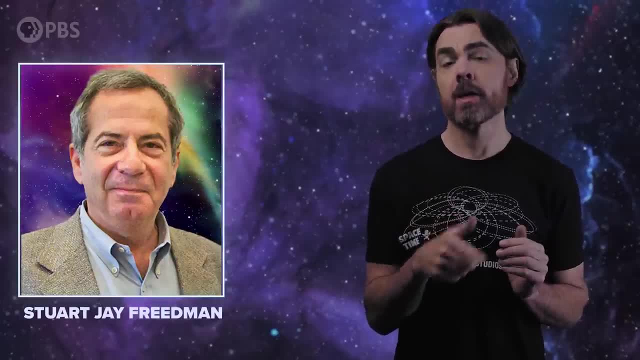 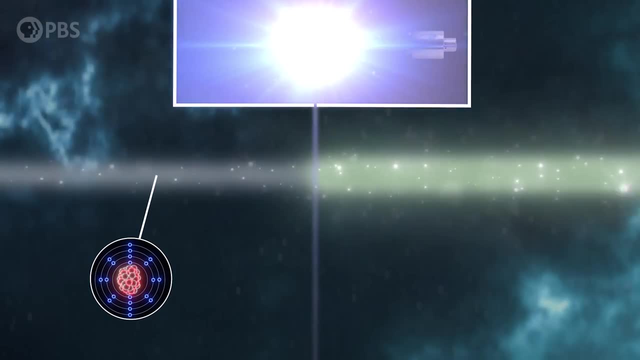 They had figured out a brilliant experiment and they were going to try it. It went like this: They blasted a beam of calcium atoms through the intense light of an arc lamp. That light excited electrons in calcium atoms to a higher energy level, and they would then. 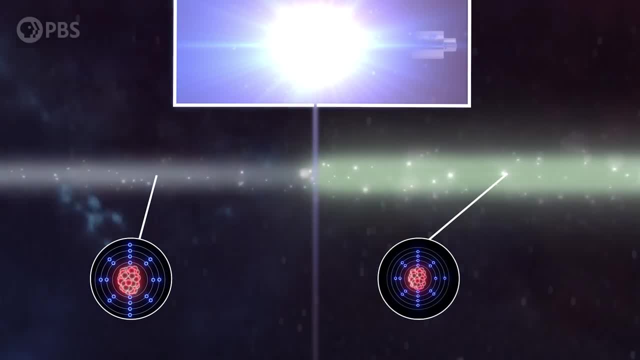 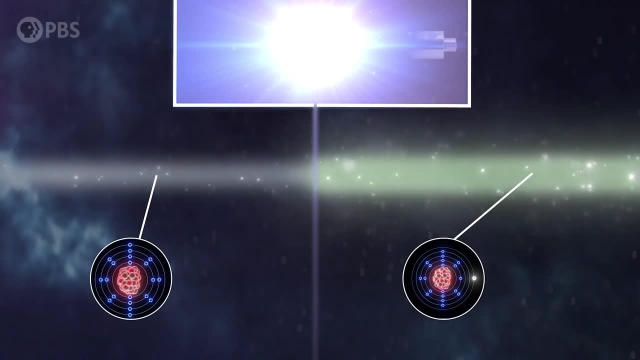 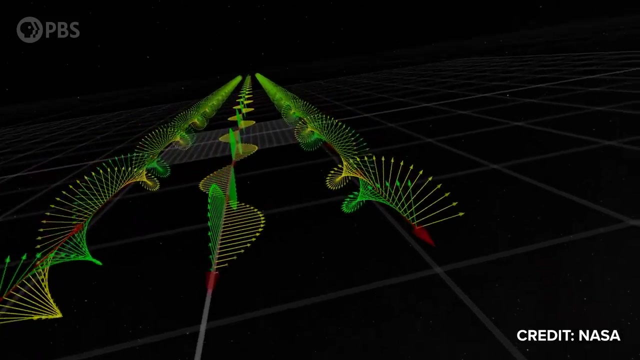 drop down again with the lost energy carried away by photons. One of the possible electron transitions was between two states that had zero quantum spin, which also resulted in the creation of two photons. Spin is the quantum version of angular momentum, Because the atom's spin hadn't changed in this transition. in order to conserve angular 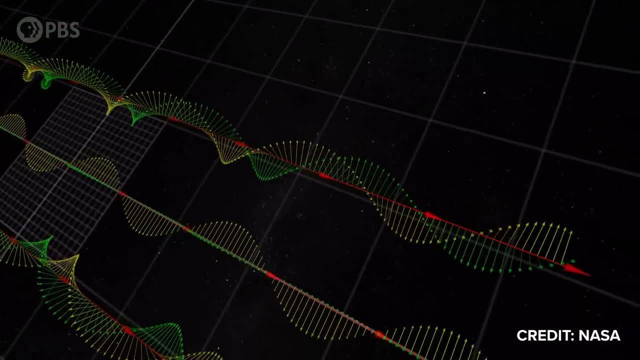 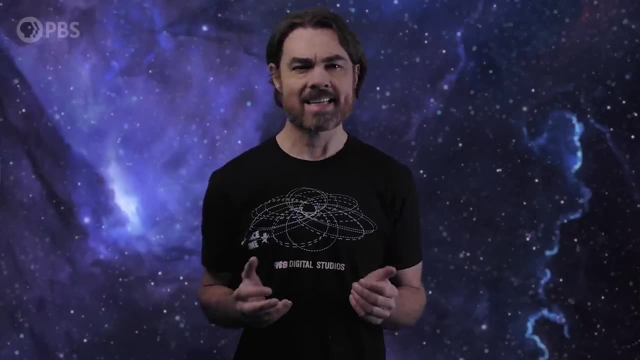 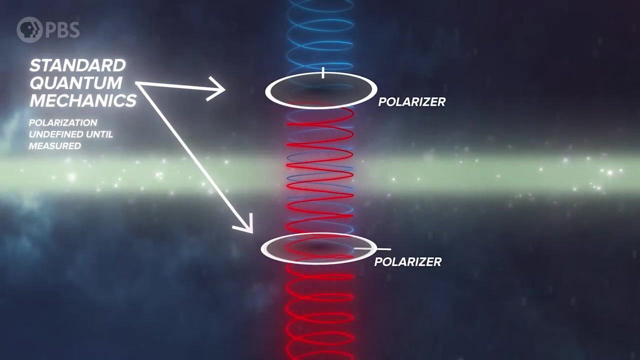 momentum, the pair of photons needed to have a total spin of zero, which translates to them having opposite circular polarizations. Standard quantum mechanics says that those polarizations are undefined until measurement, when they will always turn out to be opposite to each other. 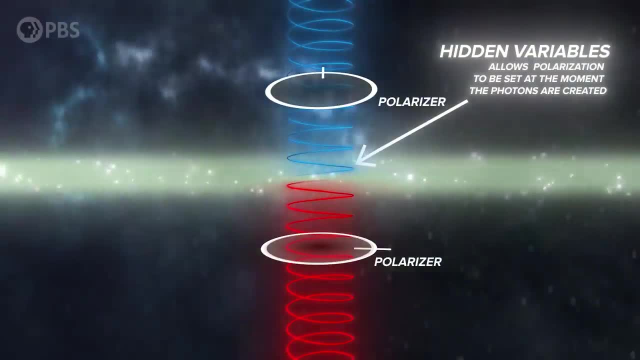 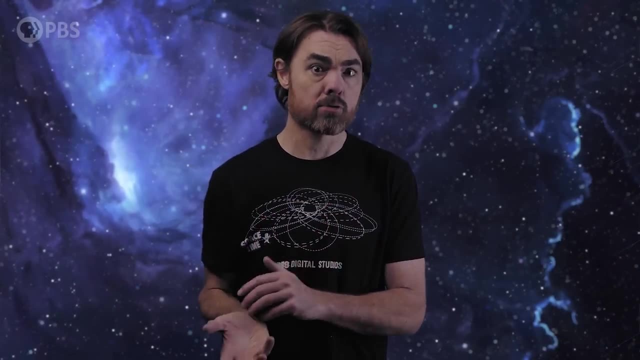 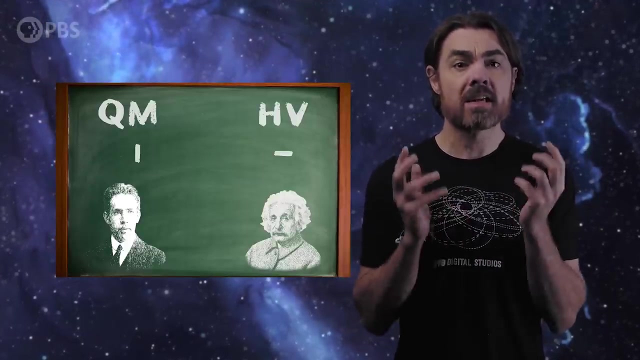 Hidden variable theories, on the other hand, allow the polarization to be set at the moment that the photons are created. By measuring those polarizations by passing both photons through polarizers, Clauser and Friedman could perform a Bell test. Bell inequality was convincingly violated in their experiment, which means quantum mechanics. 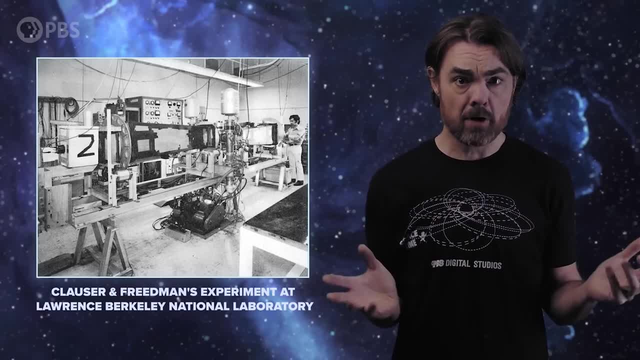 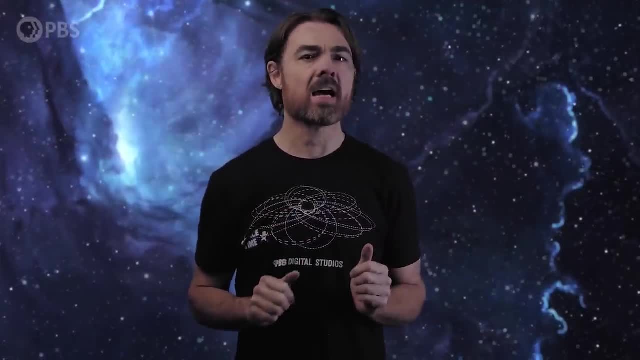 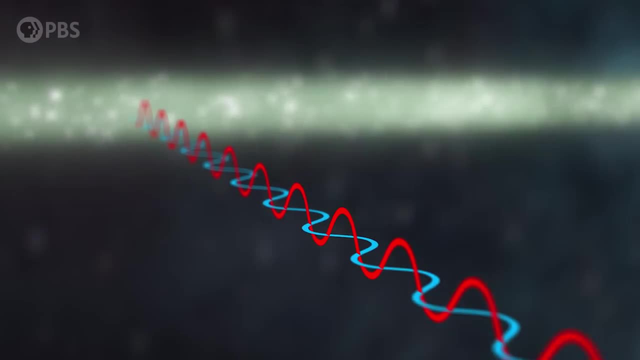 was working exactly as expected, implying no hidden variables, just as Feynman had told them. But the case wasn't quite closed. John Bell himself pointed out that hidden variables could still be a thing, Even if the Bell test said otherwise. The result of a quantum measurement depends on how you make the measurement. 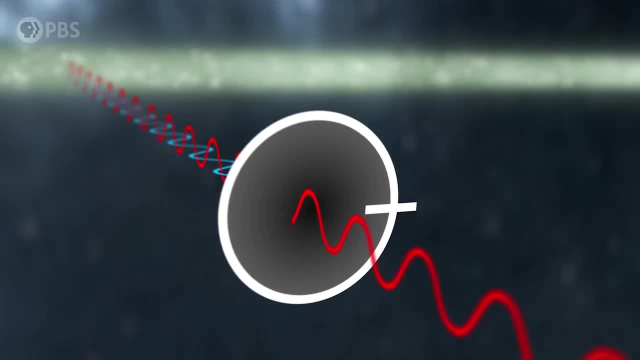 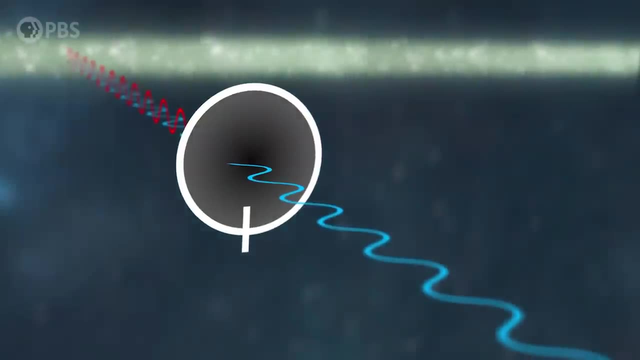 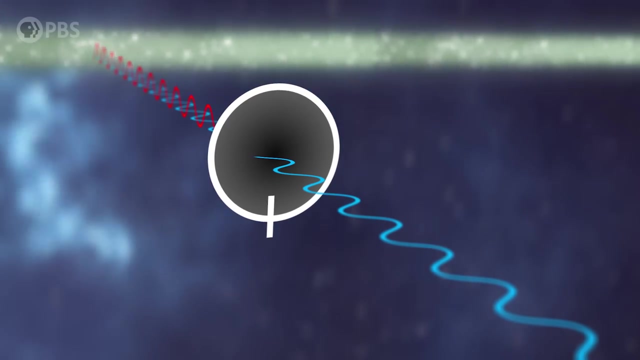 In the case of this experiment the orientation of the polarizers determined which polarizations the experiment was sensitive to. Bell's theorem, assumed that the choice of measurement is completely free and independent of the particle creation process. But in Clauser's experiment the polarizers were fixed in position through the whole experiment. 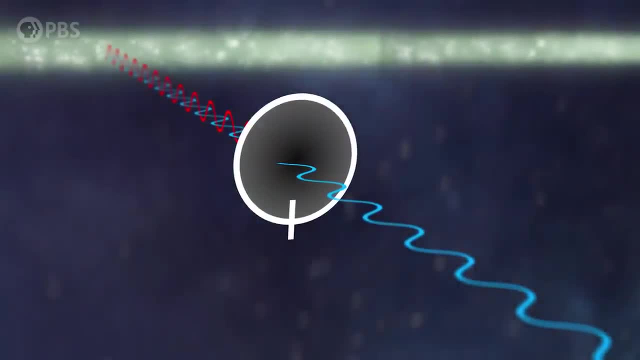 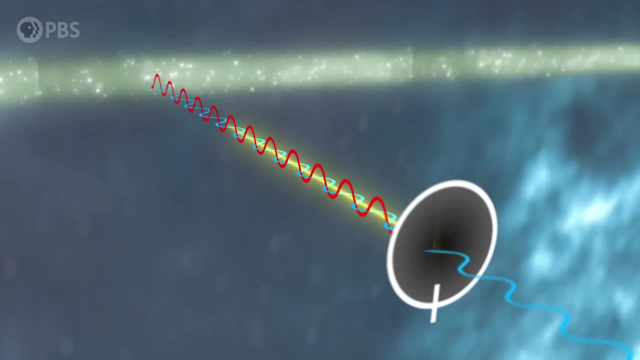 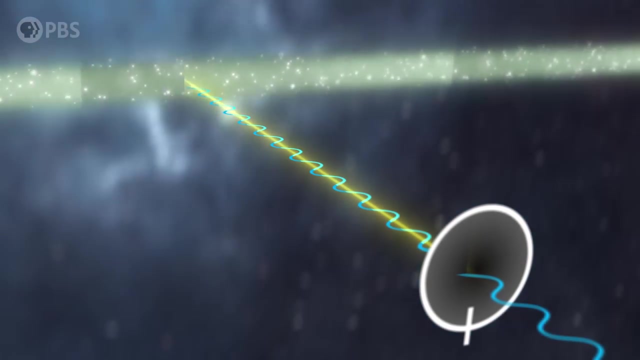 Their orientation was already designed. They decided when the entangled photons were produced. So what if that orientation had some influence on the polarization direction of the photons at the moment of their creation? Then the photons might carry hidden information about the eventual measurement direction. the 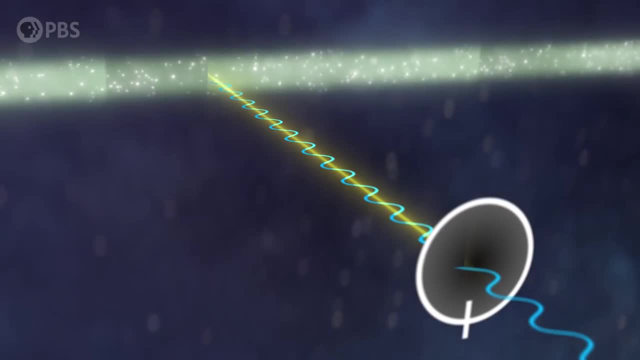 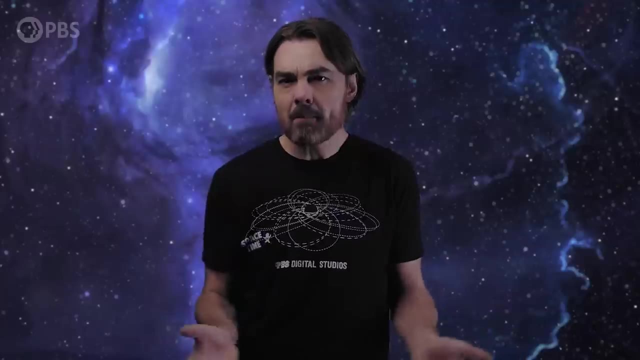 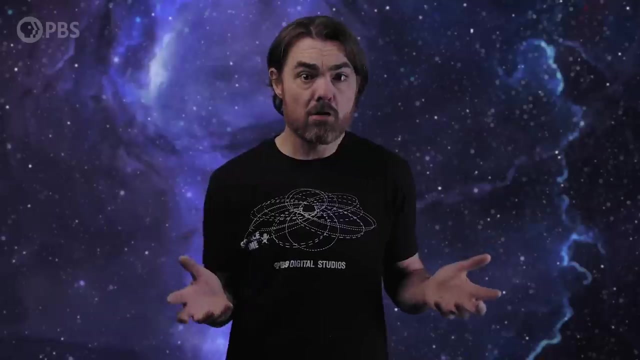 whole time and sort of conspire to look like standard quantum mechanics, even if they had real hidden variables. To close this loophole, it would be necessary to somehow set the measurement direction after the photons were produced. That sounds incredibly difficult because, in case you didn't know, photons move pretty. 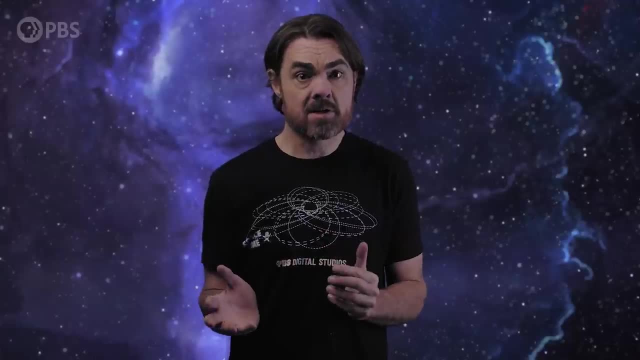 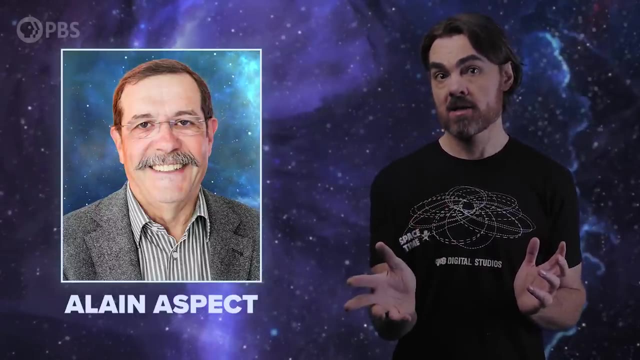 fast, But when you're a brilliant experimentalist, incredibly difficult is your bread and butter. And so we meet our second laureate, Alain Aspect. Aspect's setup was very similar to Clauser's, with a beam of calcium atoms excited by light. 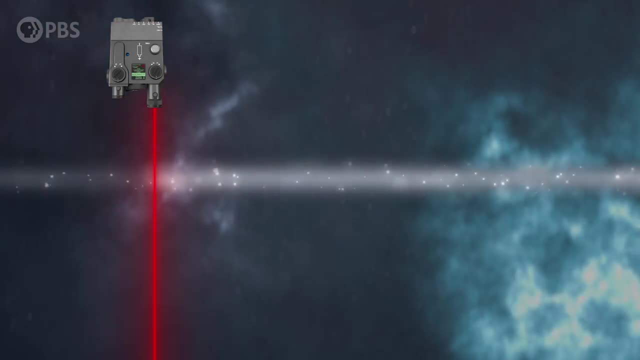 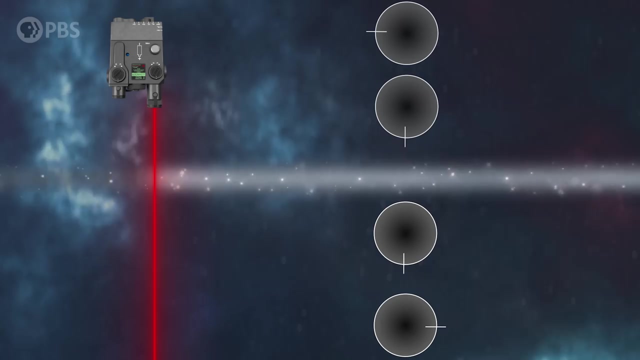 but the main difference was in the polarizers. In order to measure the polarizations, the experimenters had to use a laser. The laser was a laser beam. In order to change the measurement direction of a polarizer, you have to rotate it. 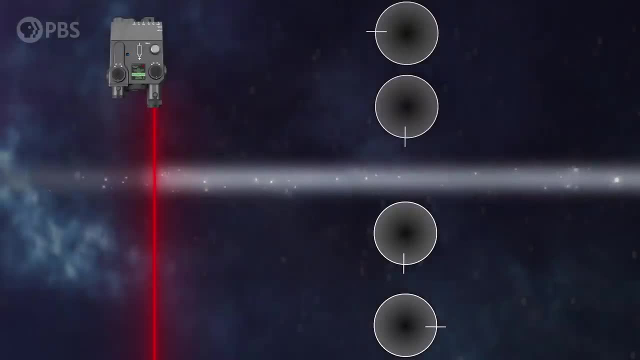 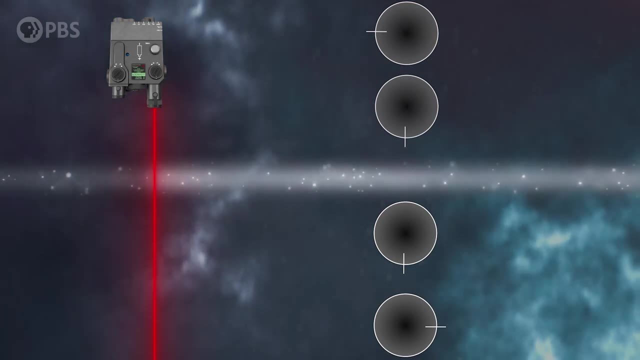 But it's kinda hard to do that faster than a photon can travel across your optical bench. Aspect found a way to randomize measurement direction without moving the polarizers at all. The trick was to use a type of transducer, in this case a chunk of quartz that bends. 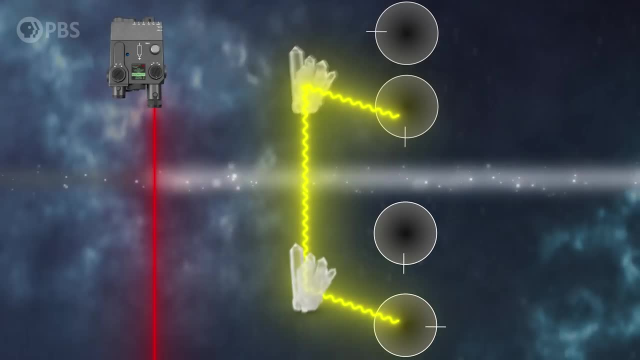 the path of light in different ways depending on whether the quartz is vibrating And that vibration can be turned on and off with an electrical device. The laser beam is a laser beam. The laser beam is a laser beam. The laser beam is a laser beam. 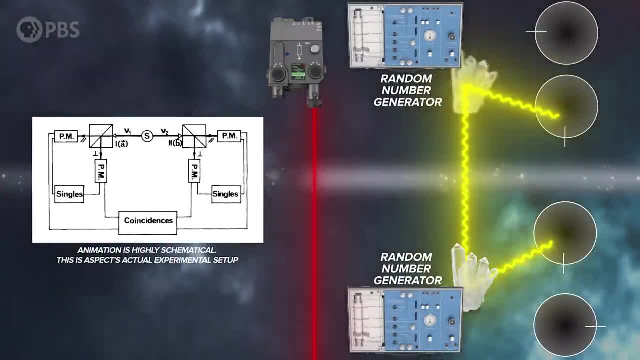 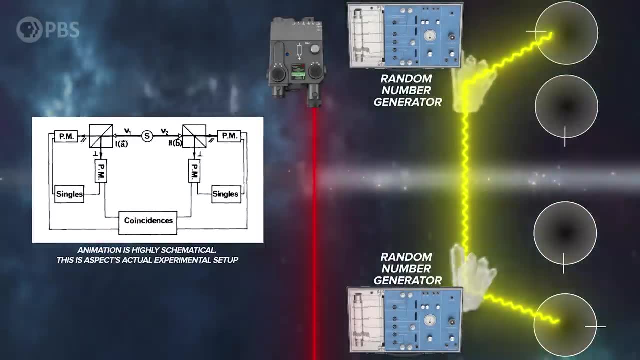 The laser beam is an electrical current That means our entangled photons could be sent to different polarizers depending on an electrical switch- A switch that could be turned on and off quickly and randomly in the tiny intervals between the creation of the photon and their arrival at the transducer. 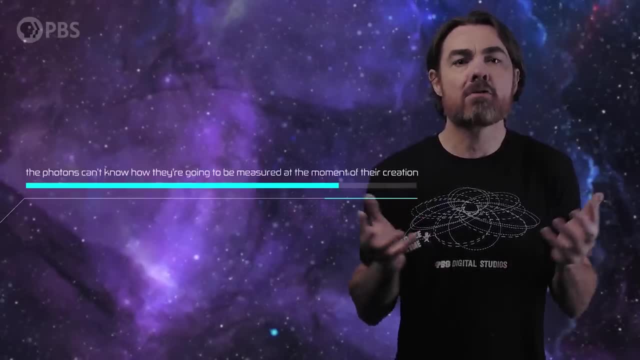 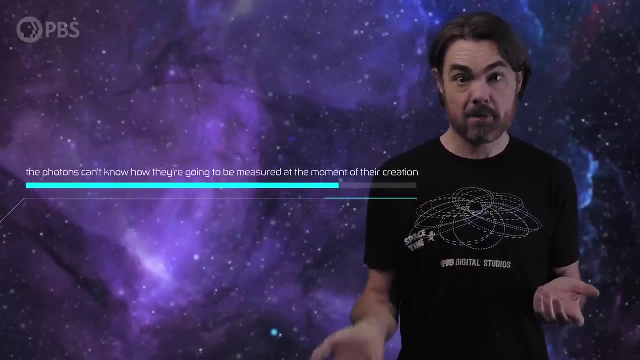 All of this means that the photons can't know how they are going to be measured at the moment of creation, which, if you recall, was a potential loophole in the Clauser and Friedman experiment. This beam is possible in light background, which will help us set up for the first step. 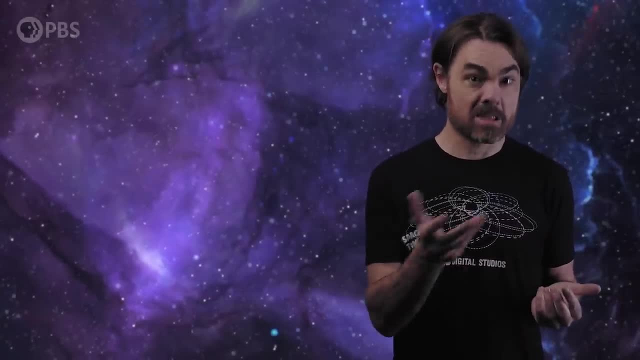 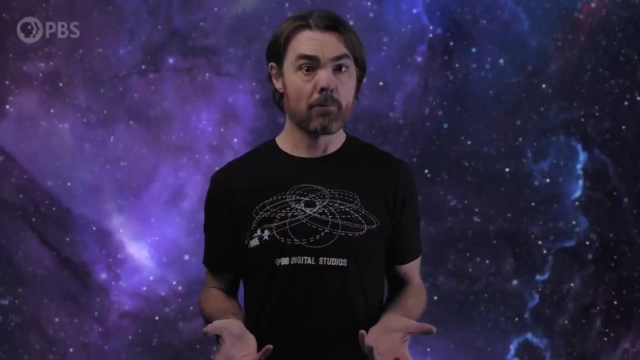 in daughterly Shahi experiment. inequalities were also violated in Alain Aspect's experiment dealing another blow to hidden variable theories. So did Aspect close the final loophole? Not quite. There are two ways that the Bell inequalities could be violated without quantum entanglement. being as spooky as Einstein feared. Well, actually these ways are still spooky, but in different ways. The first loophole I already mentioned: what if the choice of measurement is not independent of the creation of the entangled particles? Aspect's experiment seemed to eliminate that possibility by making that choice after. 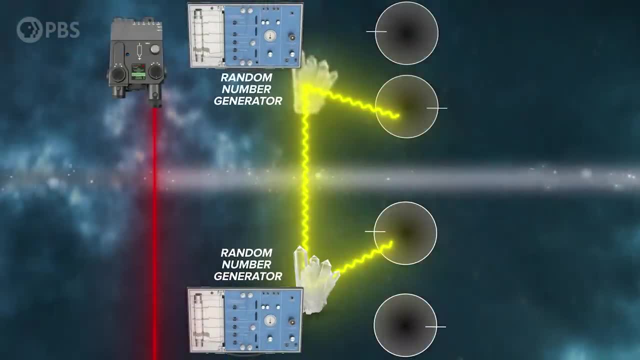 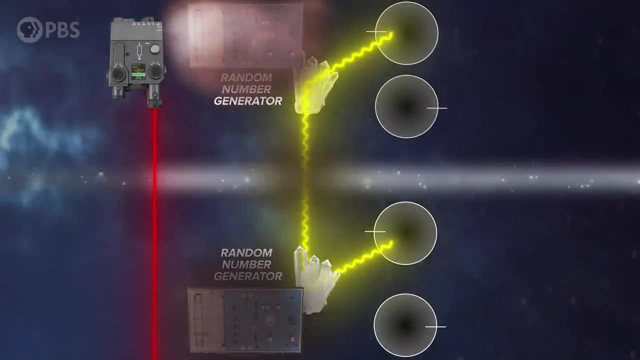 the particles were produced. But what if the random number generator controlling the transducer wasn't really random? After all, signals could have travelled to both the calcium atom and the random number generator from some common influence, causing them to conspire to violate Bell's inequalities. 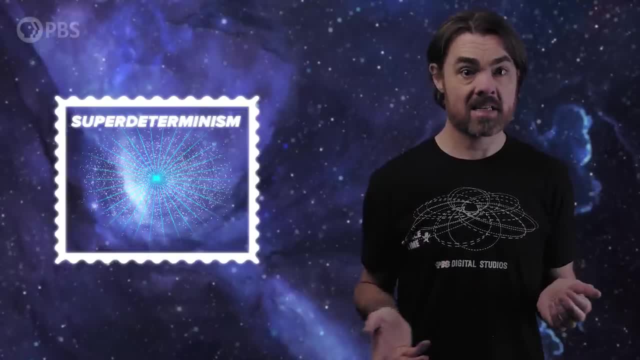 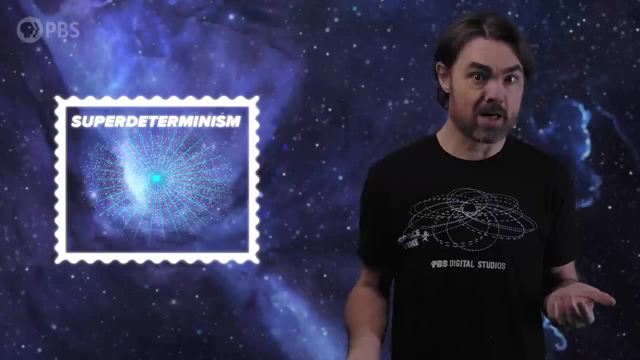 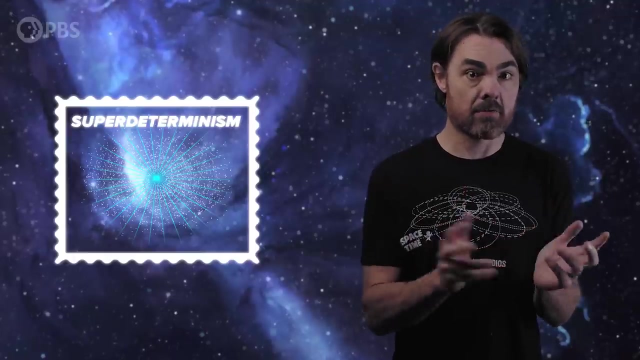 This is the idea called superdeterminism, basically stating that the particles are not only correlated with each other, but also with the random number generator or the physicist choosing the measurement direction. So, ultimately, the universe has no choice but to always hide the existence of hidden variables. 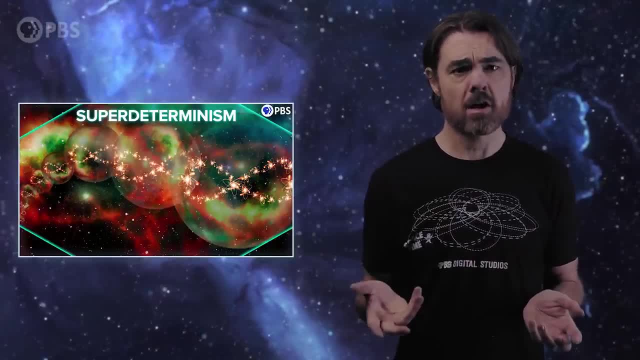 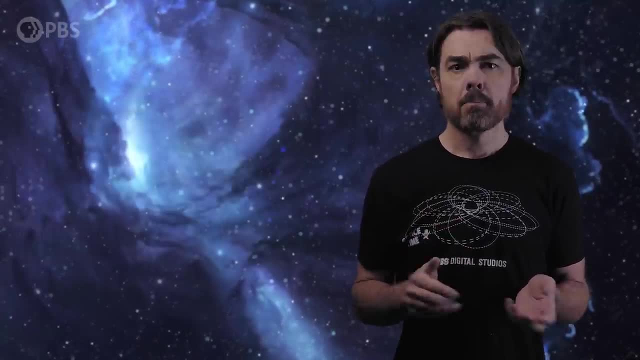 Now we've discussed superdeterminism before, so you can decide for yourself whether that's a reasonable idea. but John Bell certainly did not think that it was plausible. But even without superdeterminism there's another loophole: Bell's theorem can be used. 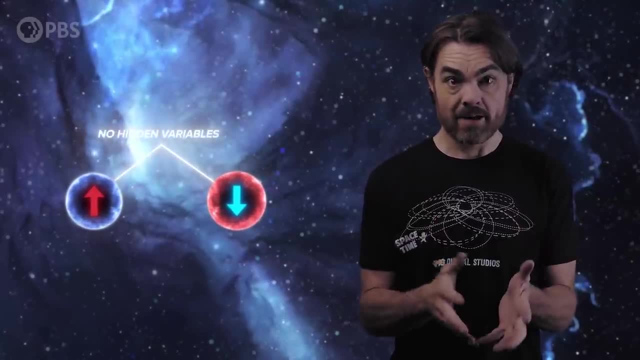 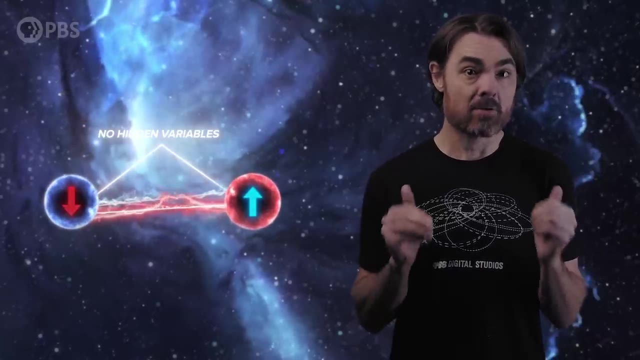 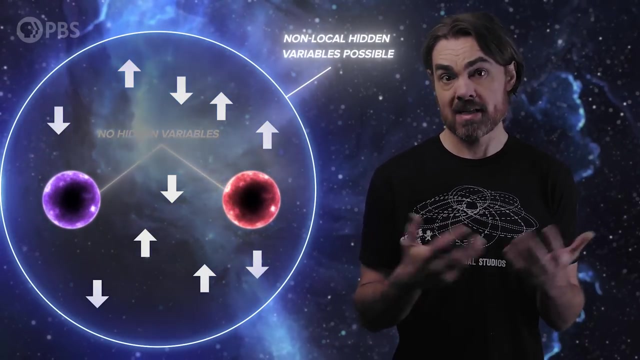 It can be used to rule out the existence of local hidden variables. It can rule out that the secret information about the entangled particles states lives in the particles themselves. That's what local means here. But there could still be hidden variables that exist in the global wavefunction of the. 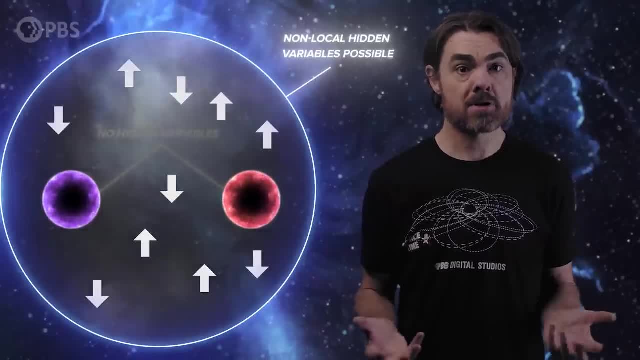 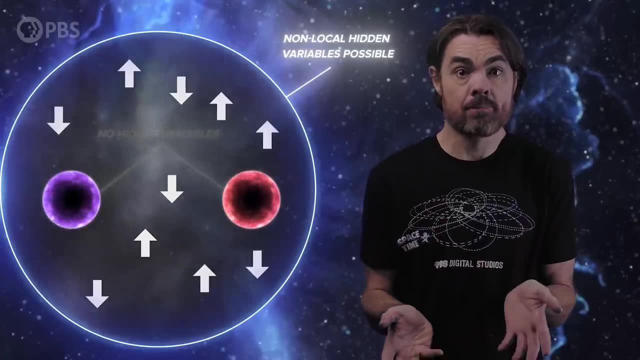 entangled particles. Clauser and Aspect's experiments ruled out local hidden variables, but that may mean they ruled out locality rather than hidden information. Any violation of locality would be considered a false. So what's the point of this? It's not just about locality. it still means that some sort of influence travels. 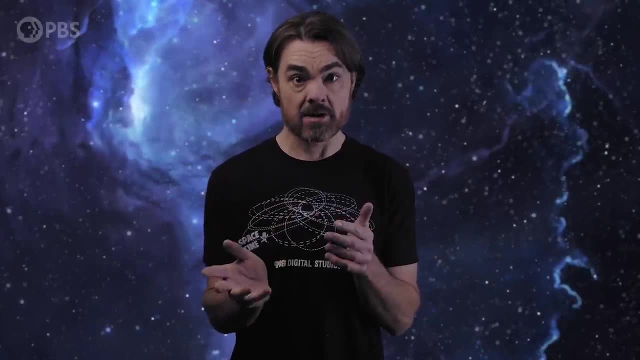 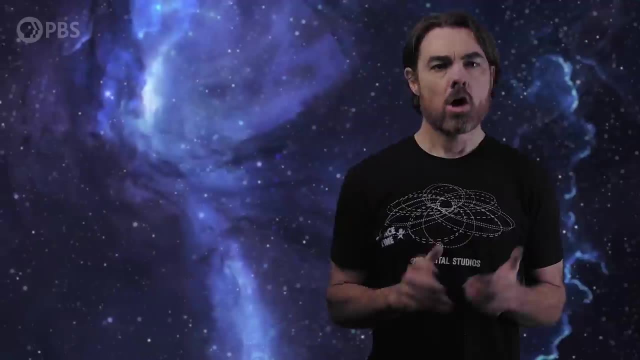 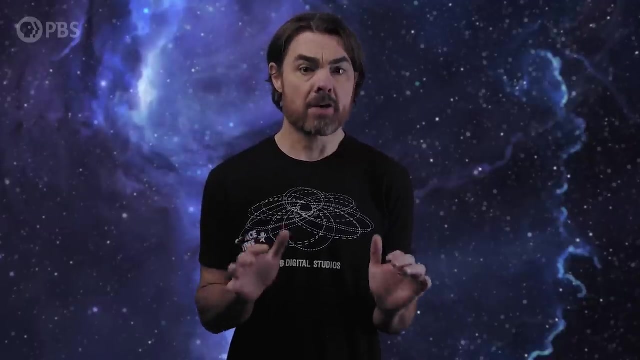 faster than light, The sort of spookiness that Einstein hated. One way or another, our Nobel laureates have revealed a universe stranger than many are comfortable with. Okay, what about our third laureate, Anton Zeilinger? Clauser and Aspect's work was all about testing the fundamentals of quantum mechanics. 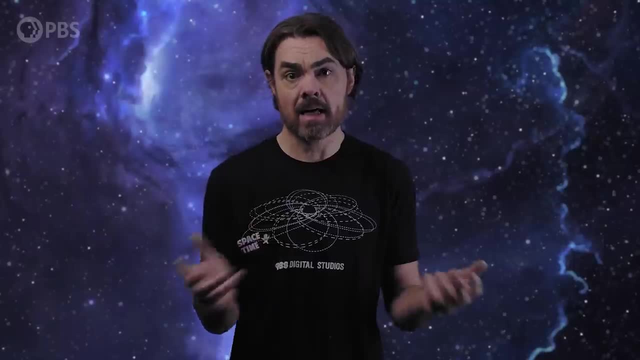 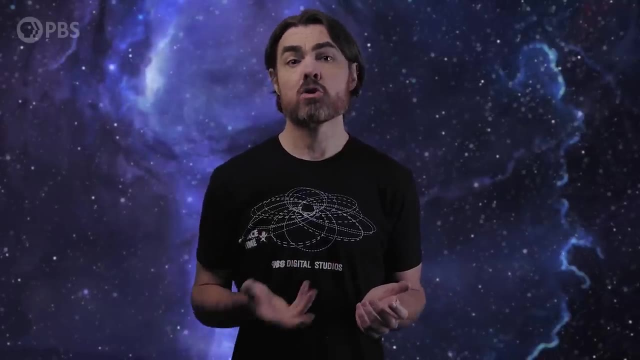 about getting closer to what its weirdness is really telling us about the world, But their efforts also led to very practical results. They and others like them advanced our ability to create and manipulate entangled quantum states, And Zeilinger put these to good use. 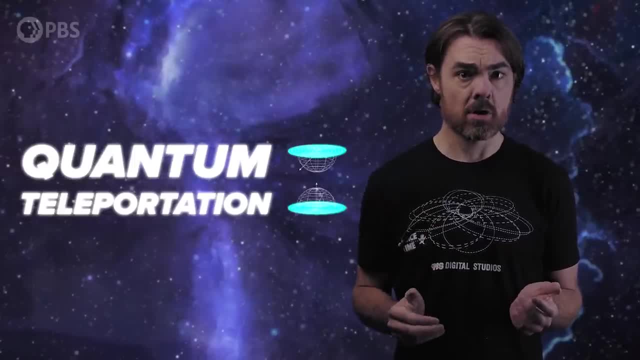 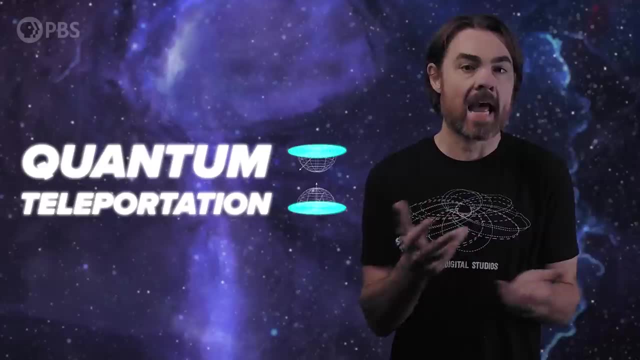 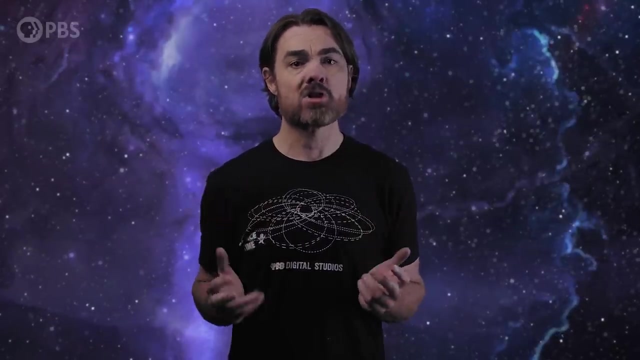 He may be the most famous for demonstrating quantum teleportation. This is a phenomenon in which a quantum state is transferred between two particles via an intermediate particle that's entangled with them both. We'll save the awesome details for another time. The important thing right now is that quantum teleportation and the corresponding ability 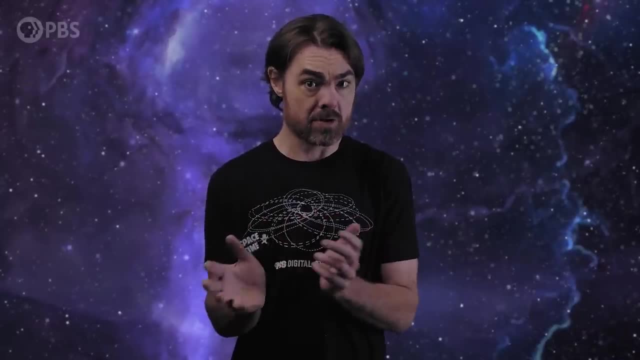 to move around. quantum information is critical for quantum quantum science. So let's get into it, Let's get into it. So let's get into it. The first thing we'll talk about is the importance of quantum computers. Zeilinger is responsible for a number of advances in manipulating entanglement and has applied 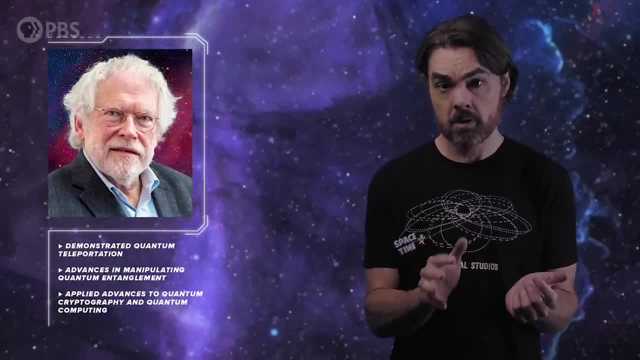 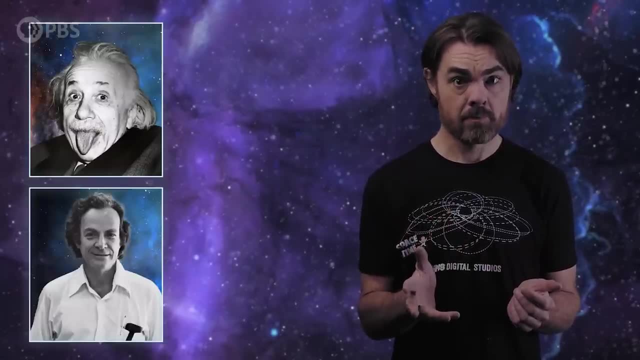 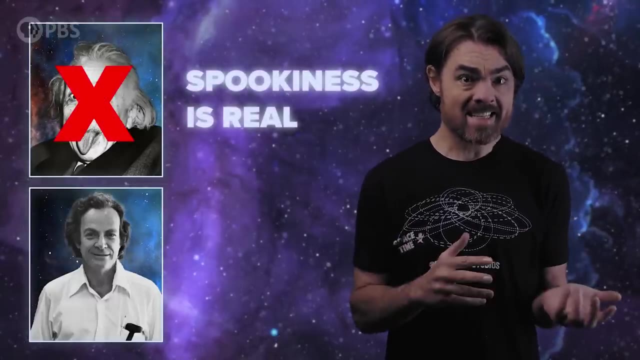 these to quantum cryptography and to the development of quantum computers. This is a rare episode of space-time in which both Einstein and Feynman were wrong. Einstein, because one way or another, the quantum world is indeed quite spooky, And Feynman was right in thinking that Clauser would never disprove standard quantum mechanics. 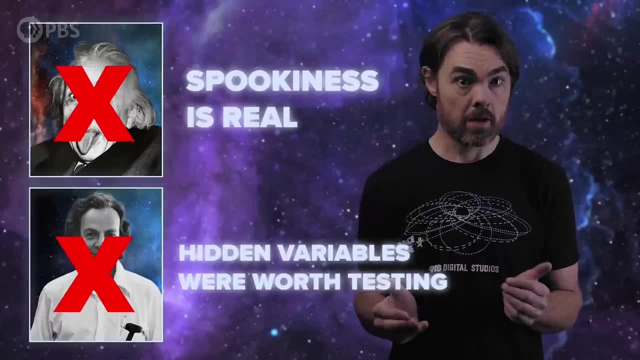 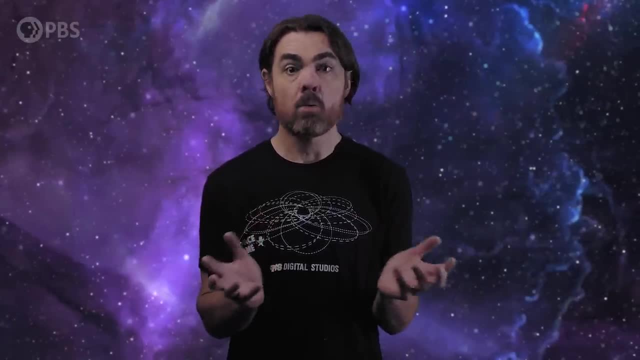 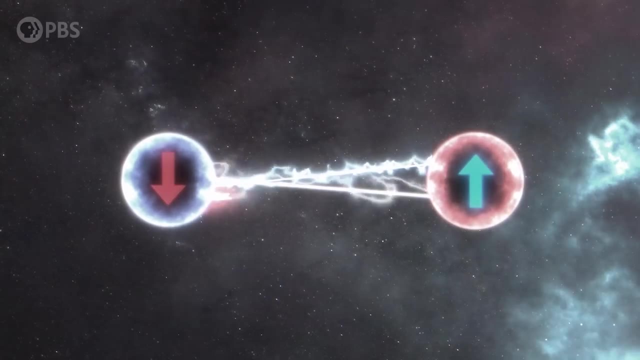 But he was wrong. wrong in thinking that Clauser shouldn't try, Because science only moves forward when we try to push its theories to the breaking point. We learn something whether they break or not, And perhaps we find technologies that will be useful in ways that no one could have predicted. 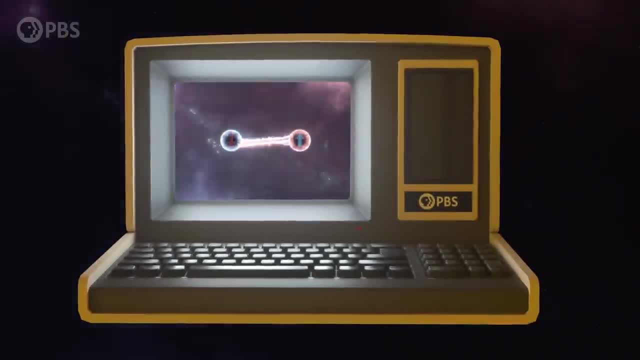 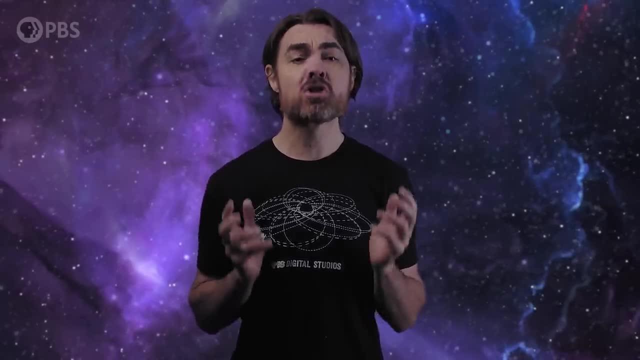 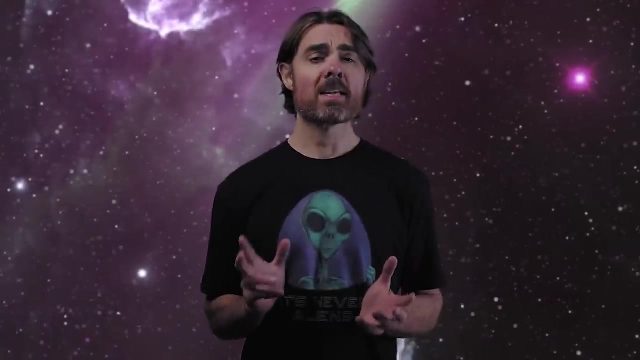 In this case, our better understanding of quantum entanglement has brought us very close to the age of quantum computing and quantum cryptography, All because a few scientists were willing to challenge the status quo and seek the hidden secrets of spacetime. Before we get to comments, two things. 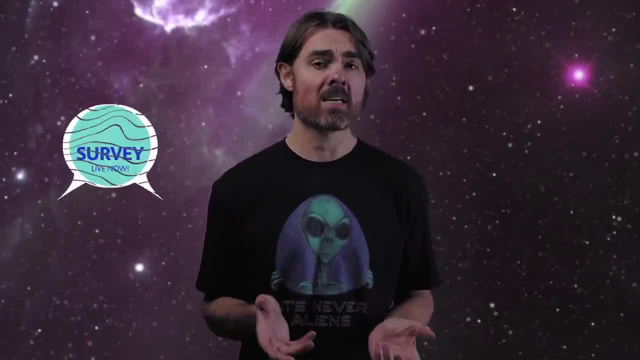 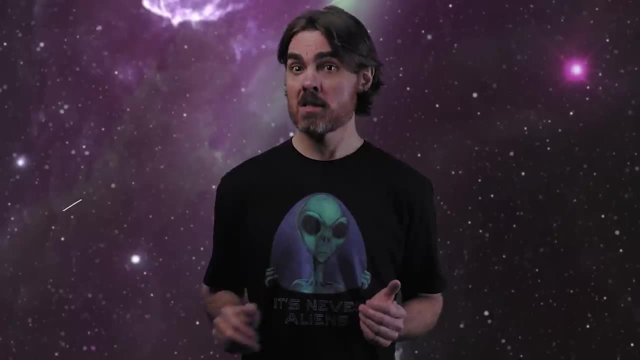 First is that time of year again where we ask you to take the annual PBS Digital Studios audience survey. The spacetime audience has always been amazing at filling out the survey, and we'd love to continue that trend. By doing so, you can help us pick out what new shows should be made and what types of 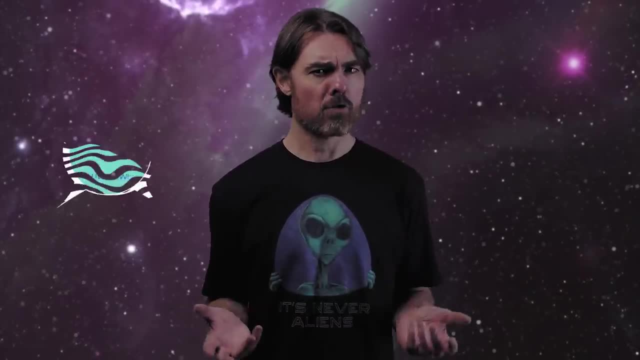 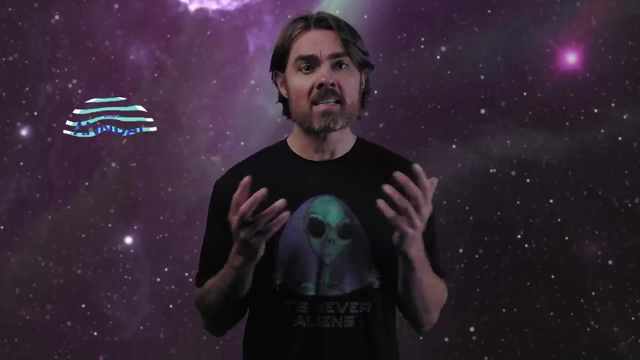 topics you'd like to see new shows cover. It'll only take a few minutes, But it's extremely valuable to us. The whole network really dives deep into the data and it helps give us tremendous insights into what you're thinking. There is a link in the description. 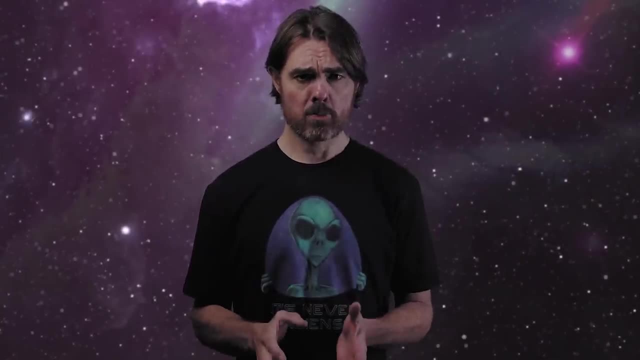 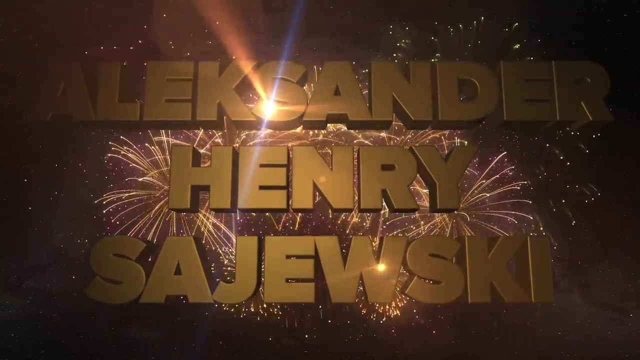 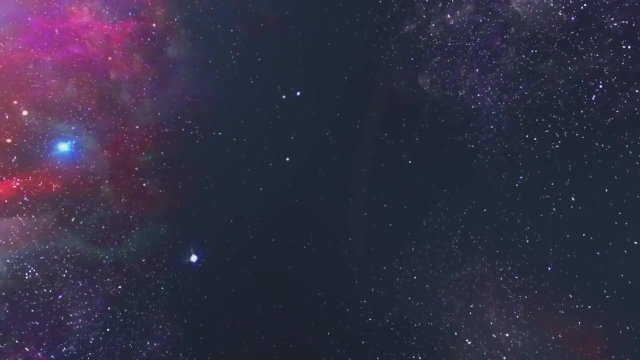 Thanks in advance. As always, we thank all of our Patreon sponsors, but today I want to give a special shout out in honor of Alexander Henry Sayeski. Alec passed away at a young age but by all accounts, was a true scientist his entire life. 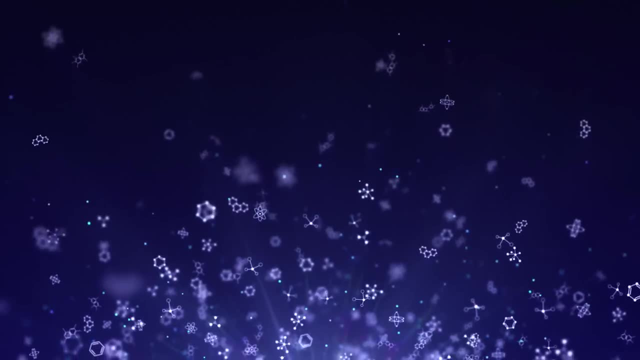 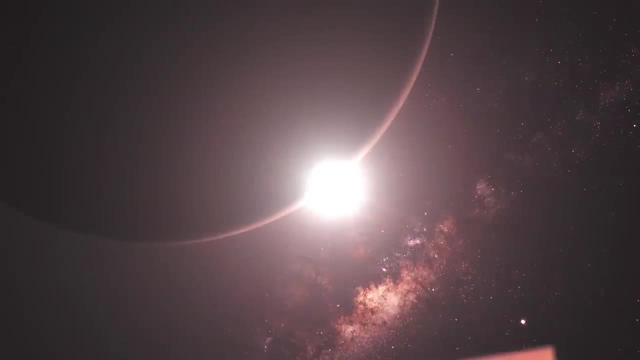 Diving into astrophysics and the sciences. when he entered college, he emerged as a professional chemist and launched into a career as a staff scientist at ALK. He was such a deep lover of the mysteries of physics and space he named his hamster. 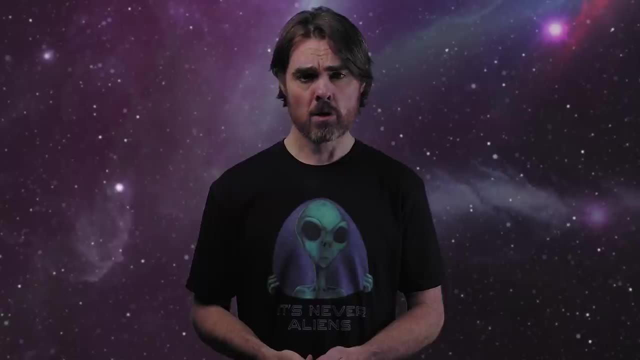 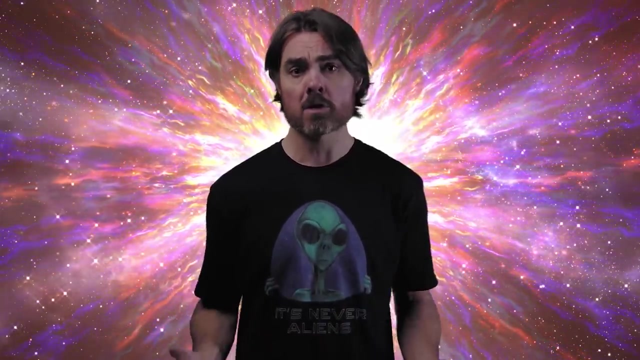 Sputnik and his fish was named Quark. So, Alec, from all of us here at spacetime, we thank you for the light that you so clearly brought to science and to your community. We hope that you find peace, Thank you. 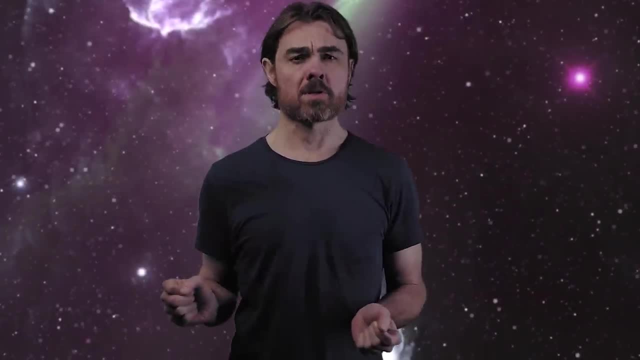 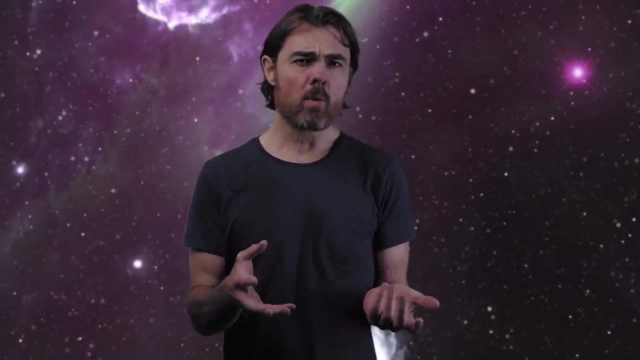 Today we're doing comments for the last two episodes. There was the one about using the sun's gravitational field as a lens to take pictures of distant planets, and then the one where we went through the entire Lagrangian equation of the standard model of particle physics. 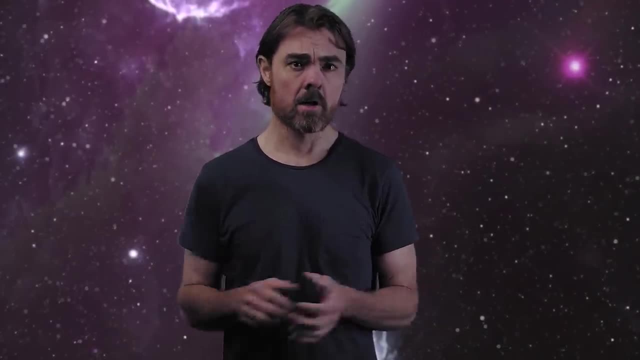 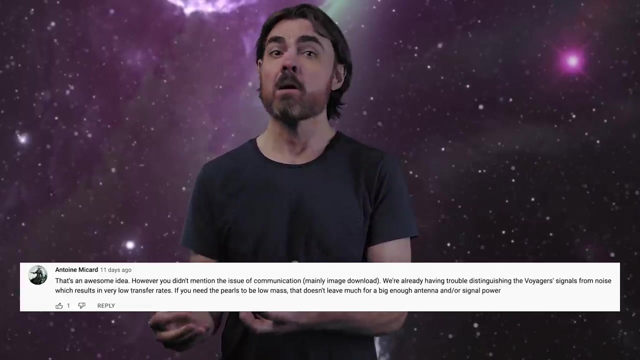 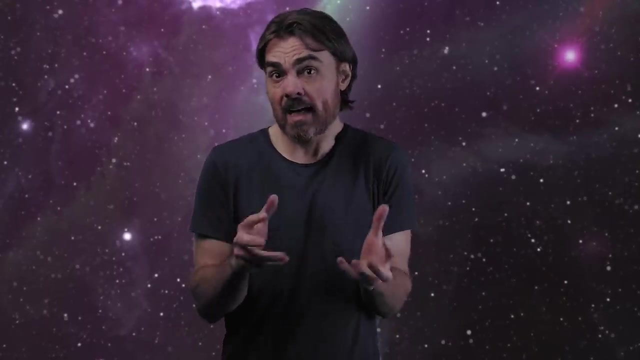 Let's start with the solar gravitational lens. Antoine Mikan brought up an important point: How do the spacecraft send their messages back home? After all, we're having a hard time keeping track of space, keeping track of Voyager's faint signals, and the gravitational lens focal range is 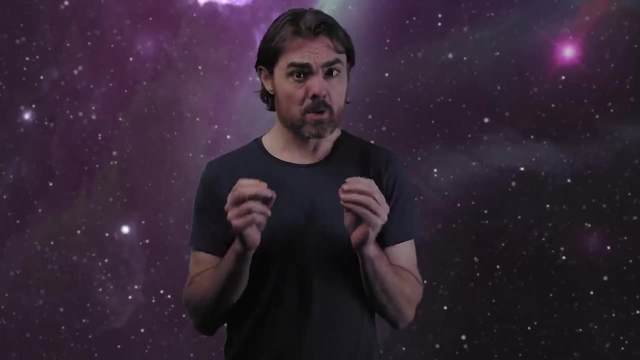 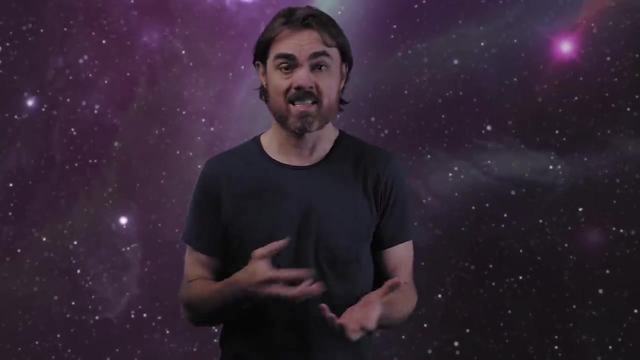 at least four times further than Voyager. While this is a real technological challenge, especially because we'll be trying to send actual images rather than simple numerical measurements and status updates, By the time these things launch, it'll be at least half a century since Voyager launched. 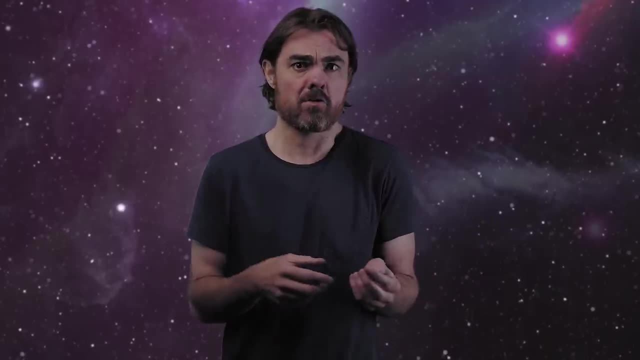 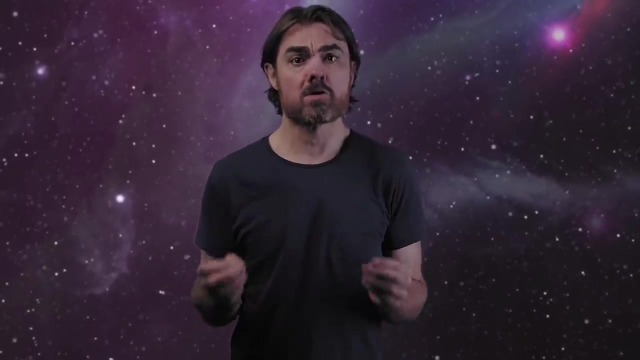 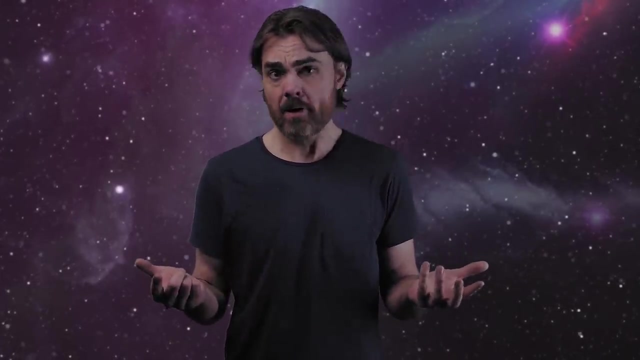 and so we'll have that much advancement in the technology of power source and power storage and transmission, And also it may be possible to use the solar sails themselves, the ones that propelled these craft to their position, as antennae, which has got to help. 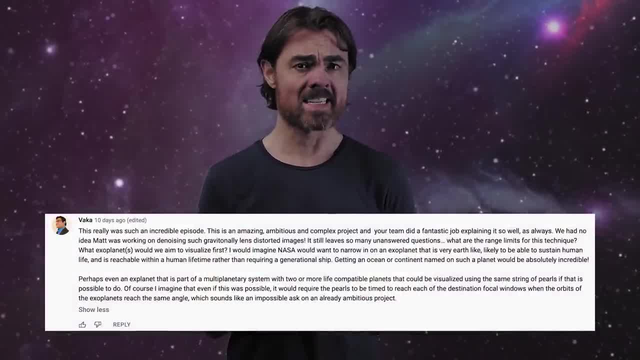 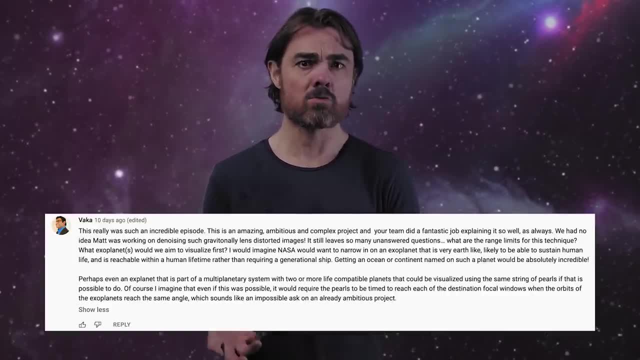 Varka has two great questions: What is the range limit for the solar gravitational lens technique and what exoplanets should we do first? Well, there's no real range limit in terms of what planets will be brought into focus in the sun's gravitational focal range. In principle, you could look at planets in other galaxies. The real limit is the amount of light you receive, and that would be too low beyond a certain distance. I couldn't find a direct calculation, but the NASA report I'd cited uses 100 light. 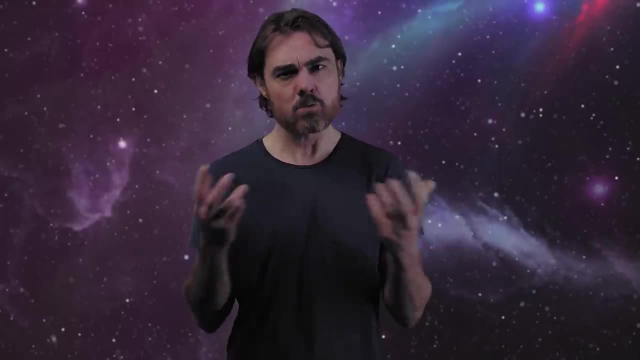 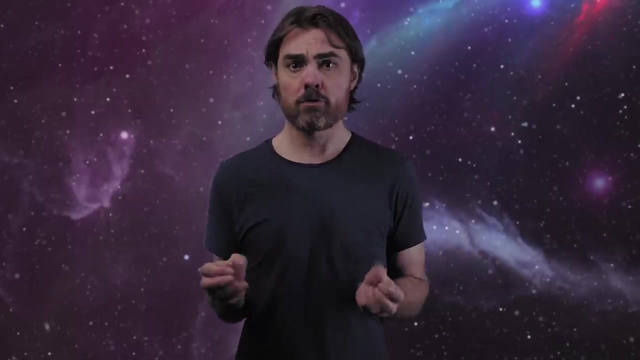 years as their canonical number. so I think the idea is that this works on the scales of hundreds of light years, but not on many thousands of light year timescales. And which planets do we do first? Well, the report talks about Earth-mass planets around sun-like stars, of which there are 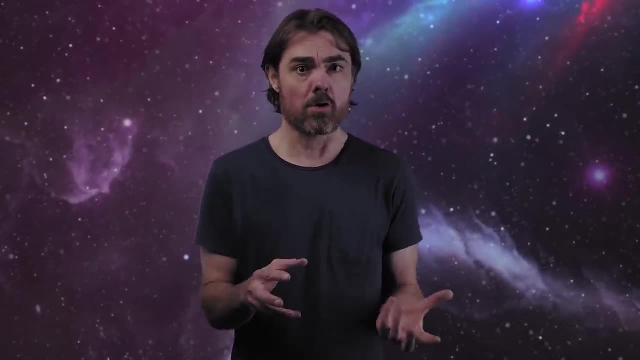 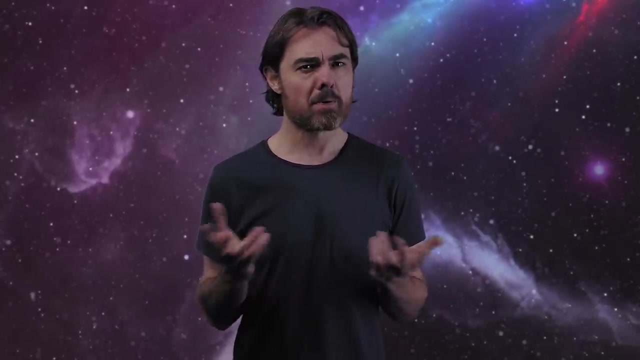 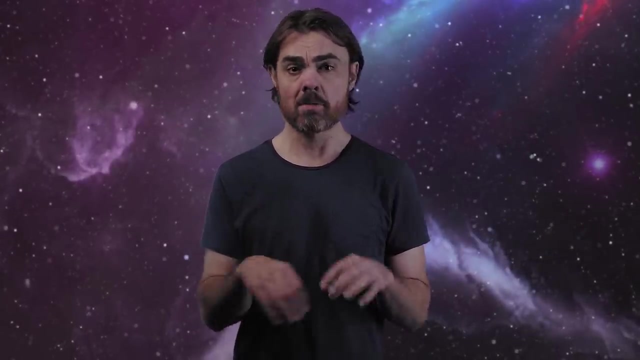 many, Maybe if we can find some that have other commonalities with Earth: Similar age system, similar heavy element abundance, maybe gas giants in the outer system, But beyond that it may be a roll of the die. Several of you commented to say that you enjoyed seeing the Standard Model Lagrangian laid. 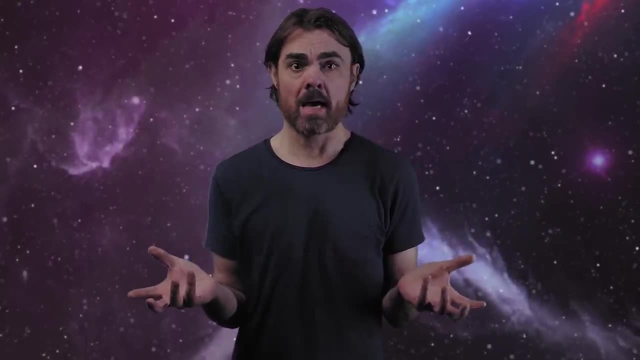 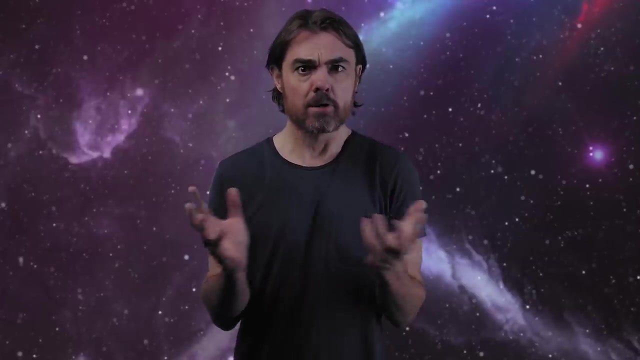 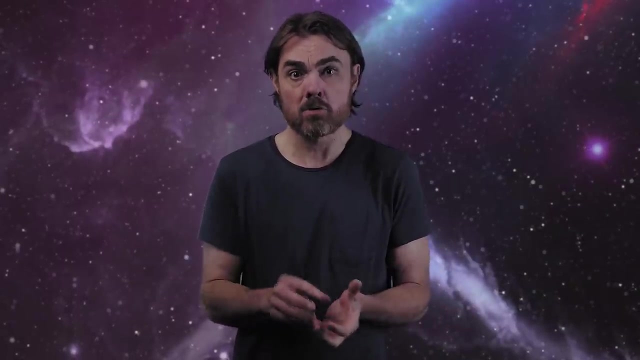 out in full, even though you couldn't necessarily follow the math. That is honestly a relief, because that episode was a bit of an experiment. There is absolutely no way to explain it. It takes several years of coursework to get close to being able to use the Standard Model. 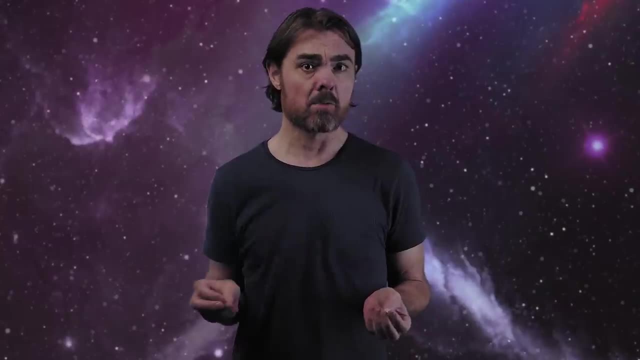 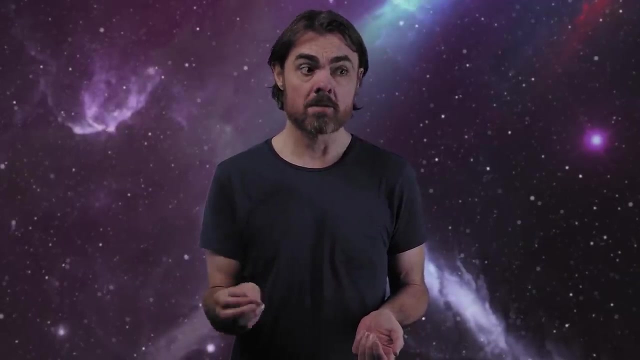 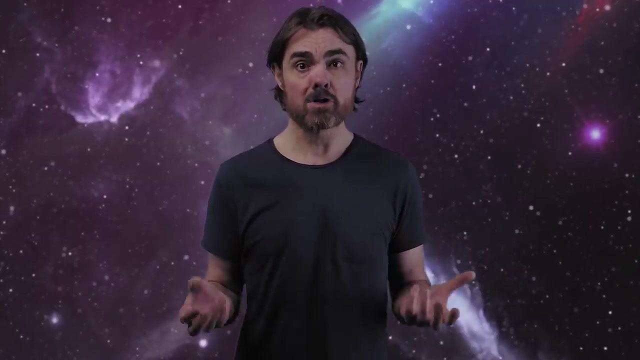 Lagrangian to do real calculations. The idea here was to give you a taste of its contents and perhaps a starting point for further investigation, So I'm delighted and relieved that you found it useful in that way. A few of you wondered whether the ghosts in the Standard Model Lagrangian might hint at. 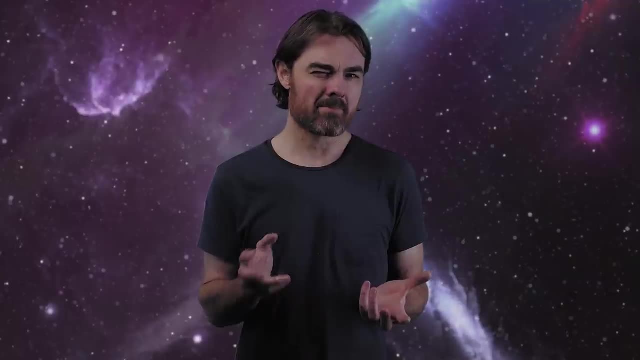 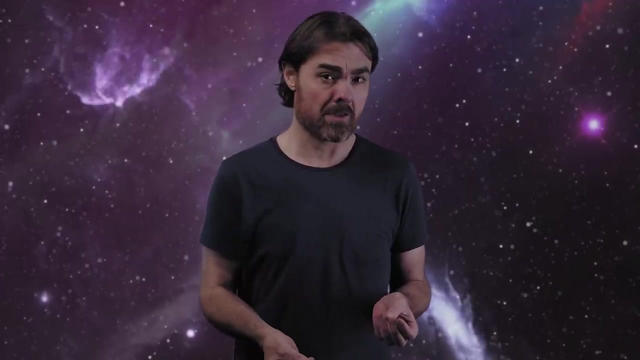 new physics beyond the Standard Model? Well, perhaps, But I don't know, I'm not sure. I think it's more likely that the ghosts could be eliminated with a more elegant formulation of the theory. Perhaps they're analogous to the spurious spaces that appear when you choose a coordinate. 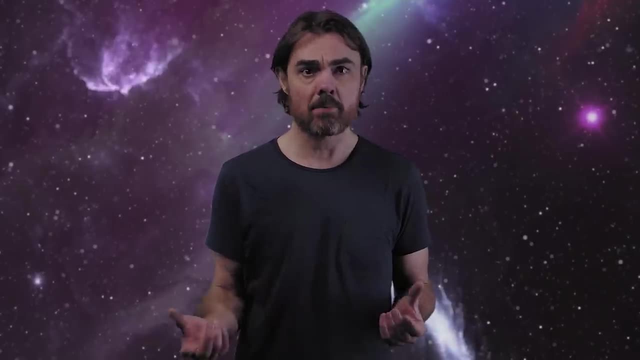 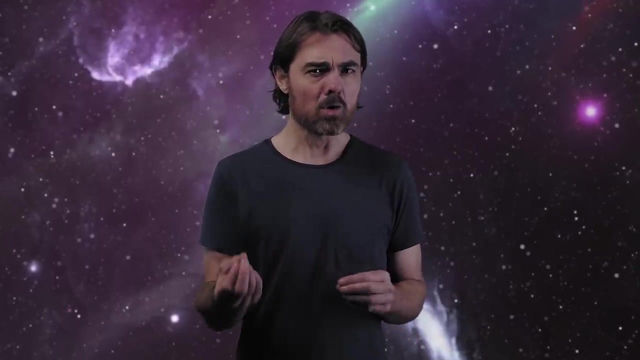 system whose dimensions extend beyond the physical world. For example, there are black hole coordinate systems that seem to imply alternate universes beyond the singularity, But more likely that's just an artifact of extending the math too far. On the other hand, I'm not a particle physicist.